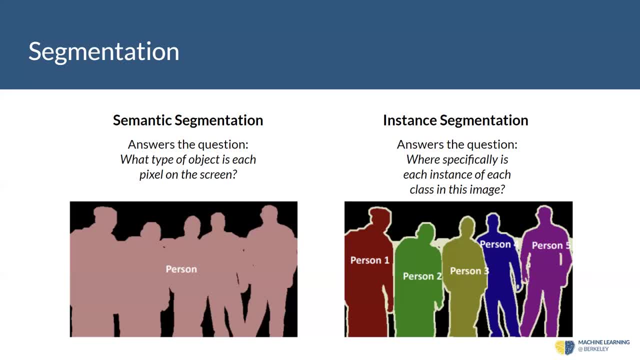 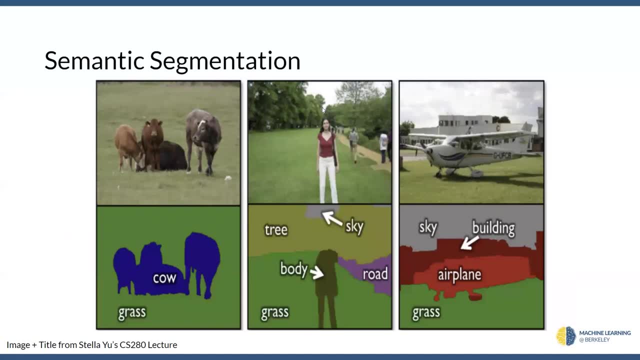 And it should be able to tell each individual dog and each individual person in the background, Etc. Again, to give kind of an example of this, It's like we have some images here. It's like we could have this image right here. 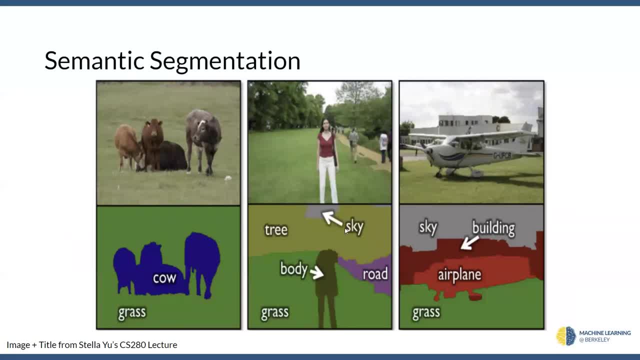 Where there's a person and grass and trees and the sky. It's able to kind of pick out all these different components And it's able to kind of segment them, Although, again notice, we're talking about semantic segmentation to start, So it can't, for example, differentiate between each individual cow here. 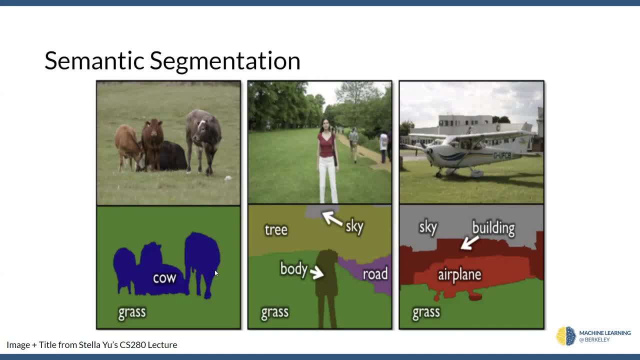 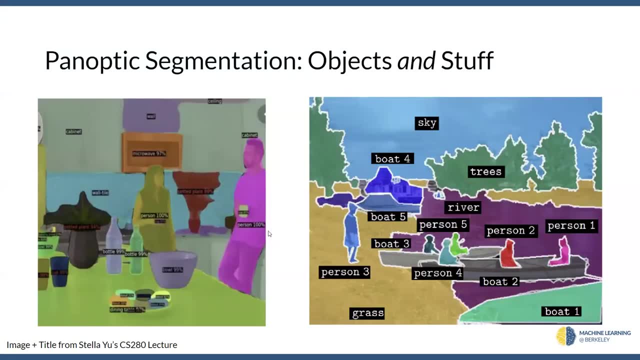 It's just classifying this as cow And kind of marking it as such. So this is what we're going to start with, But the eventual goal is that we want to be able to detect everything. We want to be able to look at an image. 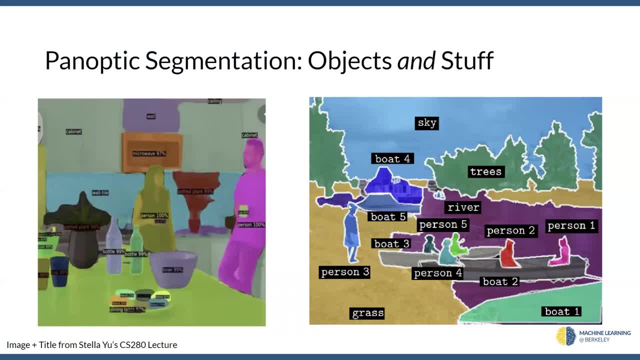 Break it down into kind of all of the different separate components. You can see this image We have: all of the different individual people are being detected differently. There's like two boats Or a bunch of boats, actually A bunch of boats that are all kind of being detected separately as well. 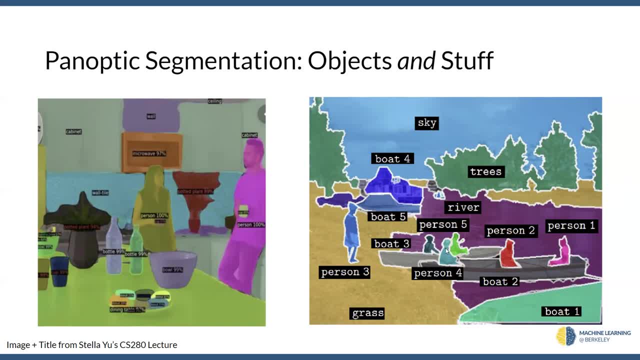 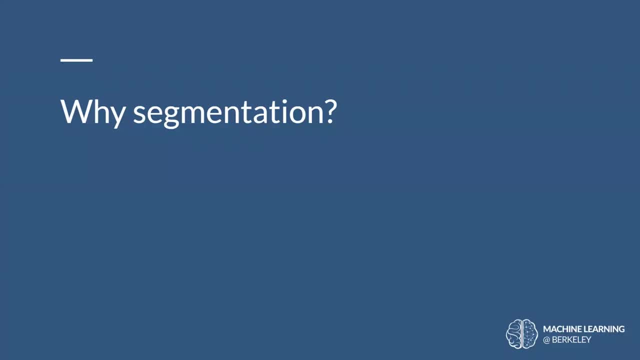 This is kind of the ideal end case. This is what we are trying to accomplish, What we would really like. So why is this useful? Because this may seem like a lot of work. It may seem kind of scary Because it seems like quite a bit of a step up from just picking a little box on an image. 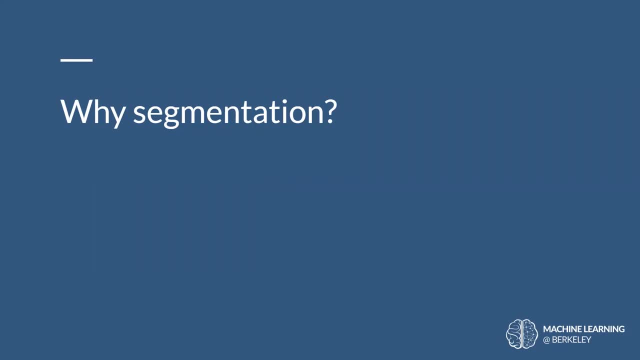 To actually classifying the exact positions of everything, Kind of separating this all out. So I guess I can hope I can convince you guys this is useful. So first of all, we have this whole idea of the gestalt principles. I don't know if you guys are familiar with this. 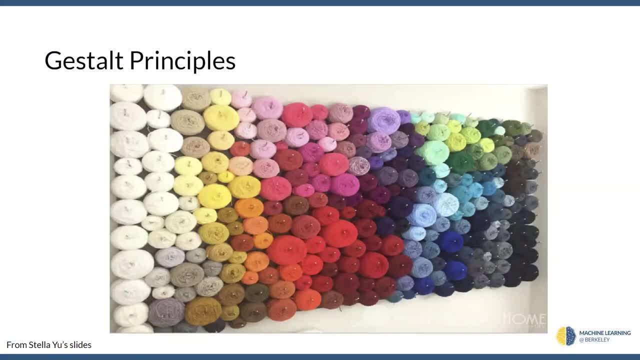 But the basic idea right, is that there's a lot of different components that go into this: How humans kind of perceive things, How they perceive objects, Right, It's like if you look at this image, for example, I think these are little balls of yarn or something like that. 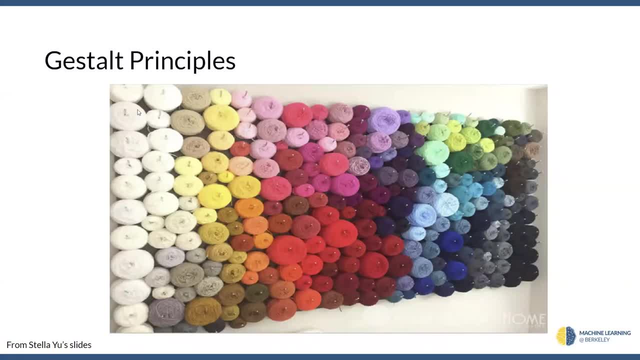 Right, It's like you know is this: you know, maybe you're seeing each of these individual bars of yarn. They all have different colors on them, But what your brain is processing is this kind of gradient: Right, It's like the whole idea is that the individual components. 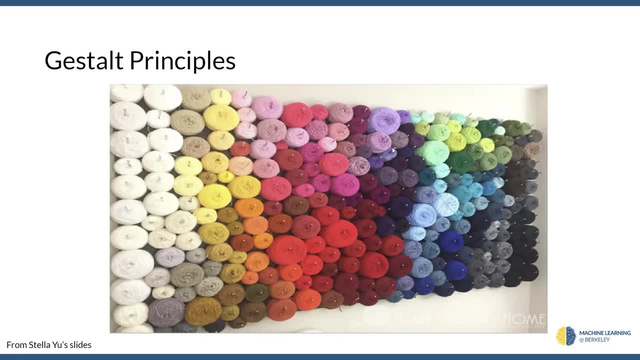 Or sorry. The whole idea is that the individual components, Or sorry, The sum of the whole image is more than just like the collection of the individual components. Right, We want to be able to actually, you know, classify and like pull all of these different things together. 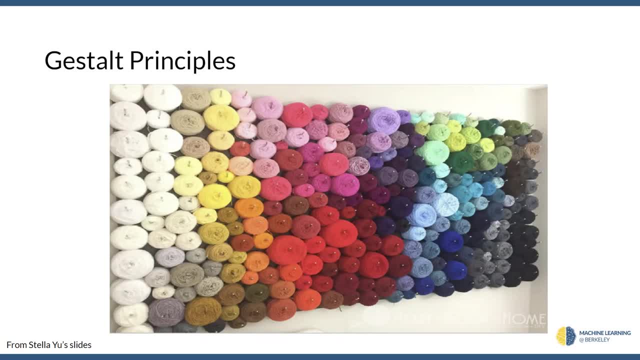 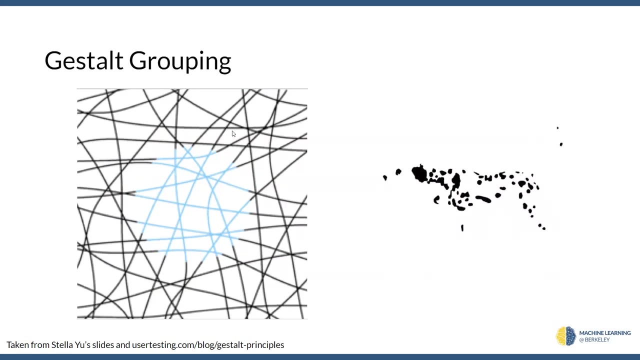 And then come up with some meaning based on that Right. So being able to kind of identify all those components of the image more specifically is really useful. So other kind of just cool aside of this that I think is kind of interesting as well is that even just determining, you know, like, what an object is or the way that we kind of perceive things, is a more general idea. 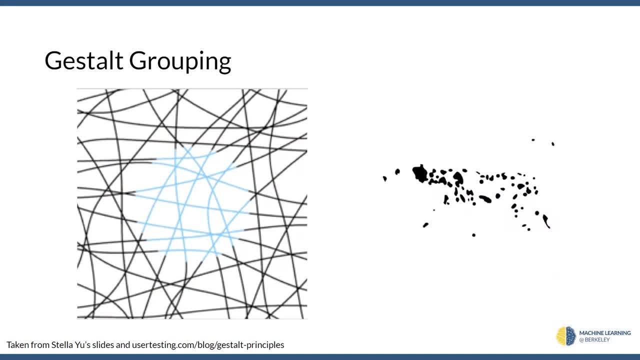 Right, It's a more challenging question than maybe you might think. it is In the sense that, like, if you look at this image Right, This is just a bunch of like weird curved lines Right Everywhere, But you probably see a circle. 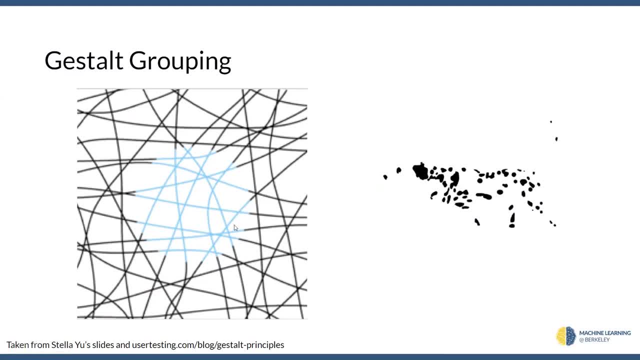 Right, Because the kind of components of the lines change color at you know an area that kind of you know happens to match that circle, Right, And so it's like how could we, you know kind of like, get these different groupings? 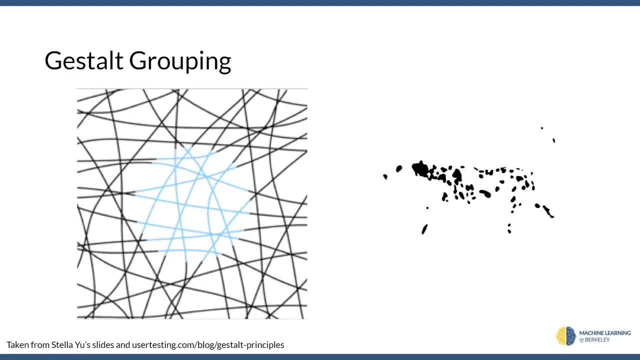 These kind of perceptual groupings. How can we kind of figure that out, You know? Additionally, you can see this example: on the right of this little you know set of weird shapes moving. I'm sure you guys all see that that kind of looks like a dog. 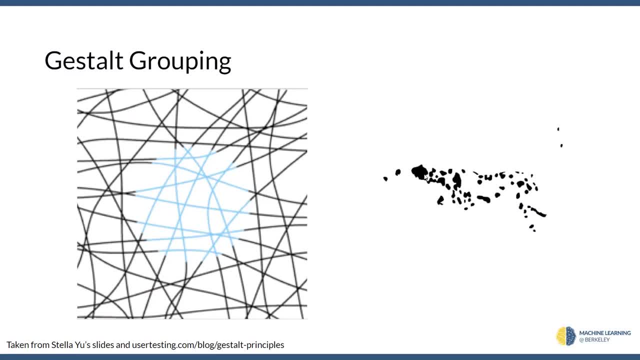 Right, Even though it's objectively like not following the shape of a dog. Right, Like if we were to, you know, talking about RCNN yesterday or Tuesday, if you guys remember. Right, If we were to, like you know, pick out the different components of this object. 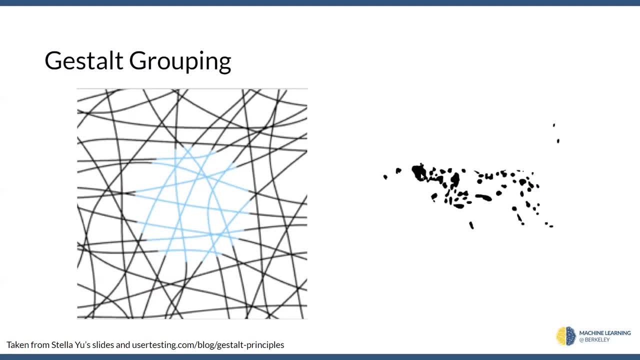 Right, And we were to, you know, like create bounding boxes on them, Right, You know a bunch of different kind of subcomponents that all kind of come together. So again, really the point of this is to kind of motivate segmentation. 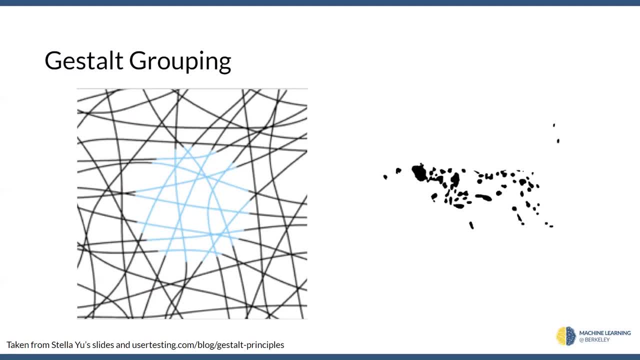 Right And why this is like a useful thing for us to look into Right. Because the idea is that if we're able to kind of identify all these different components, but we're also able to more generally- you know, connect different, you know classifications, or kind of do larger level, you know segmentation, this becomes a really really useful ability to have. 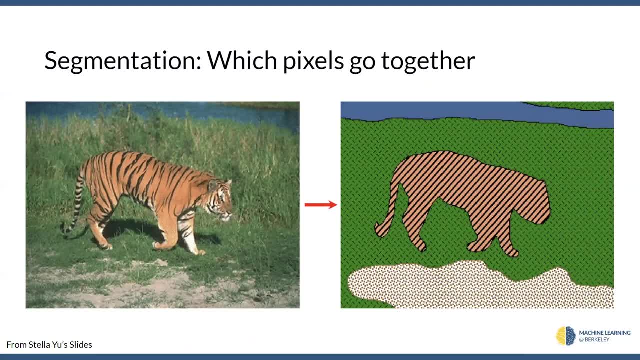 So again, yeah, So, yeah, So, yeah. So this is just really. there's a lot of like really abstract speaking, But the basic idea is just: segmentation is telling you which pixels go together, Right, Like taking an image, telling you these two are pointing, or the same thing. 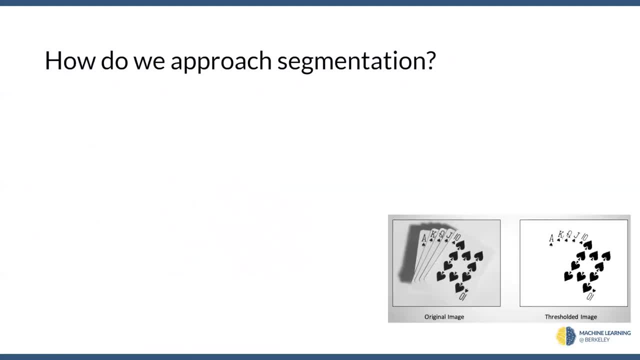 Right, These are different. So how do we approach segmentation? So there's actually a component of this that we brushed over. last lecture We actually referenced segmentation in the RCNN section again, When we were talking about region proposal. We were actually saying that we will use some magical, classical, you know, region proposal method that will just magically look at an image and propose to us boundaries that might be good regions to classify on. 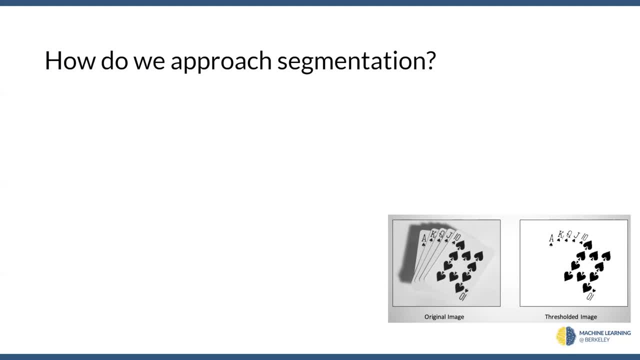 Right, And so we're actually going to take a look at, like what that actually means, how it's kind of implemented. There's obviously lots of different methods to this, But the simplest possible way that we could kind of approach this is as follows. 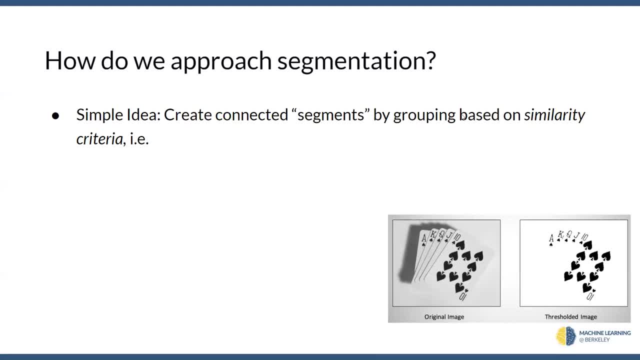 So, first of all, We connected segments by grouping based on some sort of similarity criteria, Right? So if we have, you know, like this image right here, Right, Maybe we want to, you know, group together potentially the cards. 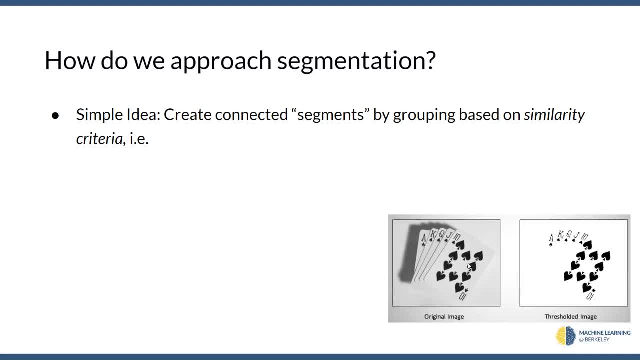 Or maybe we want to group together the you know individual components, Like you know little spades on this playing card. Right, It's like we want to group together visually distinct objects on a maybe not so distinct image. So let me just 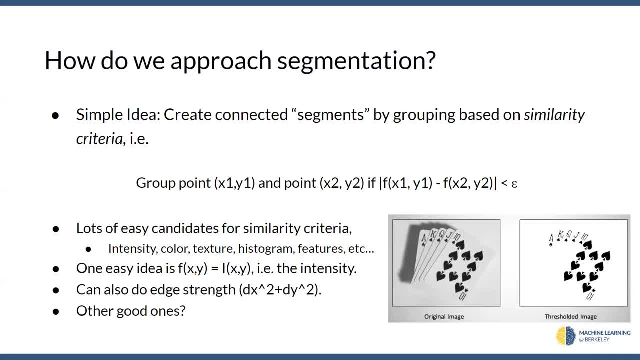 Yeah, There we go. So one way to approach this is that we can essentially define some function by which we were to group pixels together Right As in, if we have some image Right Like, let's say, we have this image down here. 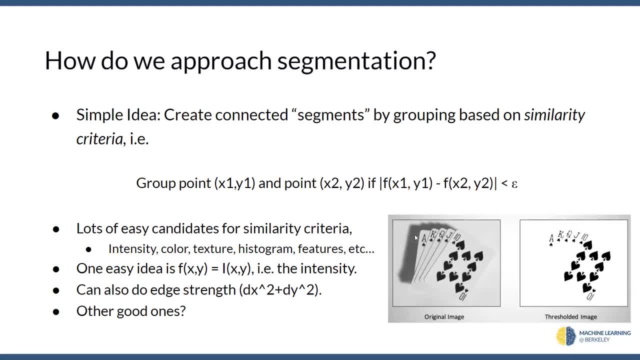 And we pick point: you know this point right here, Which maybe is X1, Y1. And then we pick- you know a point next to it- X2, Y2.. Right, And then we pick point: Return some like similarity criteria. 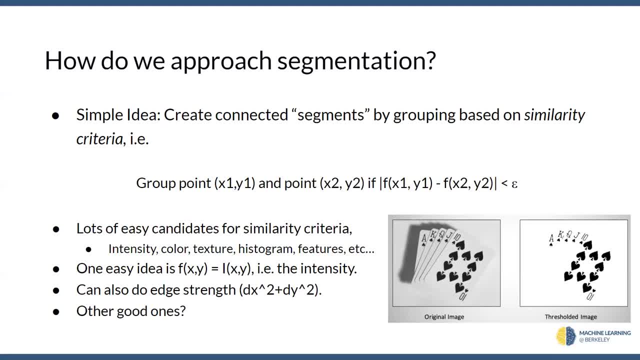 We can essentially say: if the difference between those two, if those two pixels are similar enough to each other, Their difference is below some epsilon, Then we group them together. Right, And so this is like a very simple, kind of classical approach to this problem. 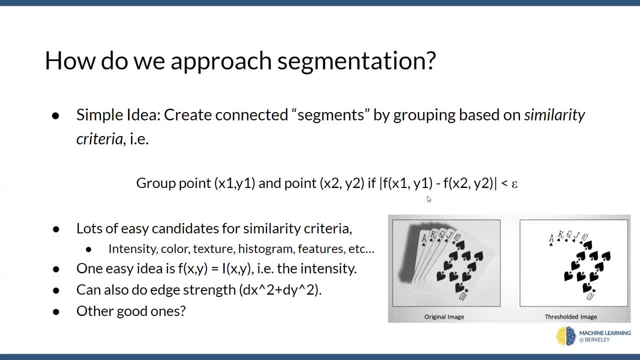 And there's a lot of different similarity functions Or like metrics that you could use to measure similarity. A classic one is just, you know, intensity, So like the brightness of a pixel. That's not the technical definition, But you can think of it as: 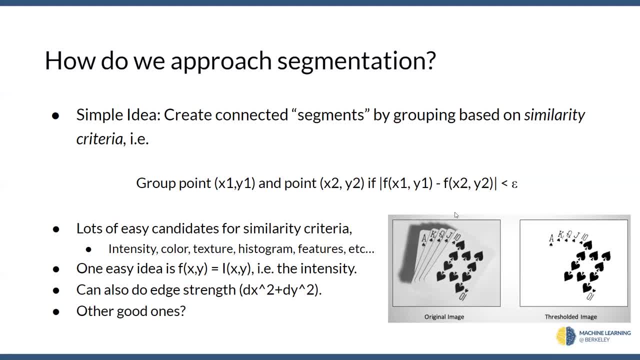 Right. It's like the intensity of a pixel is like how kind of bright that color is Right. So, for example, If we look at you know, this pixel right here And this pixel right here- Right, They are pretty similar in color. 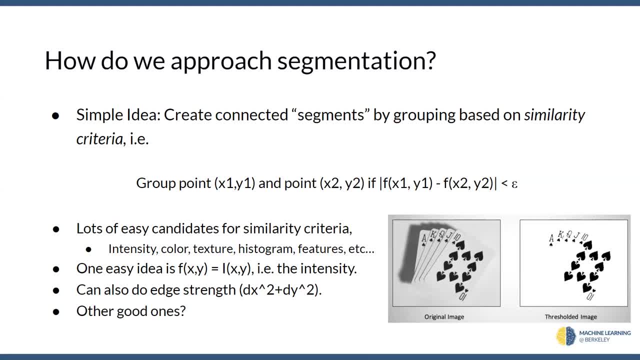 But they're not too. I mean, they're pretty similar in color, But they're a little different, Right, And so we would kind of merge those two pixels together In the sense that we would consider them part of the same group. 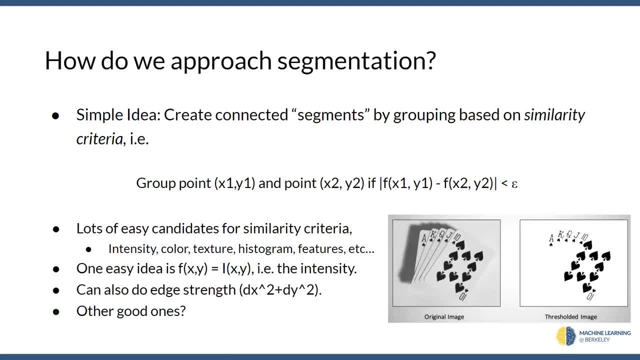 Right, And then kind of, you know, flood bill outwards here, Right, And then maybe we'd get an image that looks like this thresholded image on the right, Where essentially you know, there's the white section, is like all of the kind of pixels that have been grouped into this one, you know, collective segment. 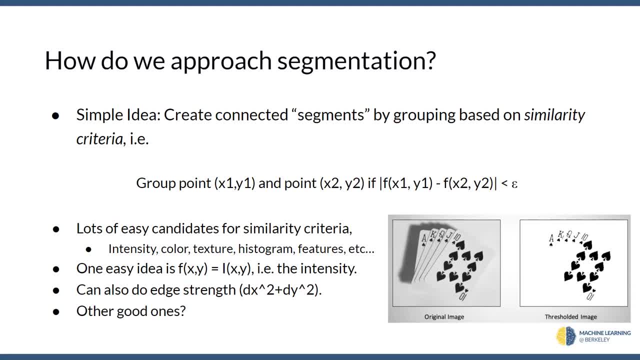 Right. So there's lots of other ways to kind of approach this, But the idea is that's kind of, I guess, a very, very basic, classical approach to this problem. So we're going to look at the fixed algorithm. 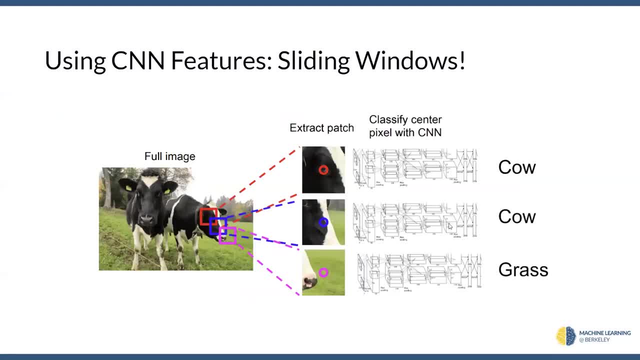 Now we're going to look at some- you know, newer- maybe deep learning- approaches to this. So one way that we could kind of do segmentation- that's a little bit more interesting because it's learned as opposed to a fixed algorithm- is we can go back to that sliding windows idea that we talked about on Tuesday. 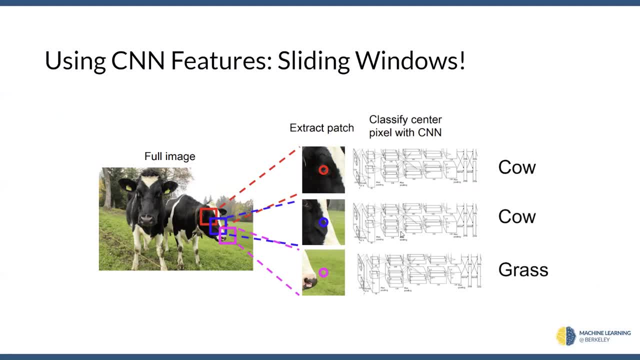 Right, Except this time, instead of doing sliding windows in an attempt to classify a bounding box, what we can essentially do is we can slide windows across the image And then we can have, for each- You know- slide of the CNN, That current box. its only goal is to classify the middle pixel of that box. 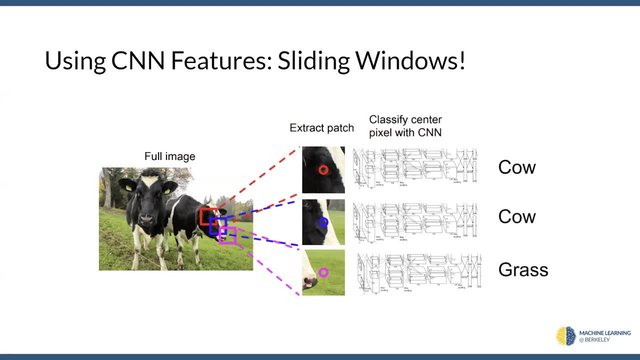 Right In the sense like if we had, you know, this red square down here. right, it's running classification on this patch of the image And then it's outputting what it thinks the middle pixel is Right, And so what this allows us to essentially do is is we can run this CNN sliding windows. 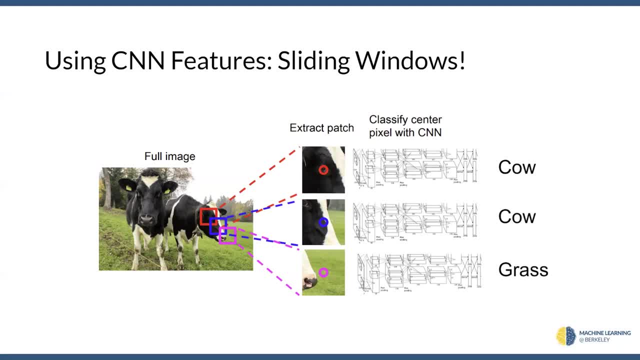 Right, And so we can have a window across the image And every time it outputs it'll output you know what object that should be a part of, And then on our output image, like our segmentation map, we can just write that you know value to the corresponding pixel. 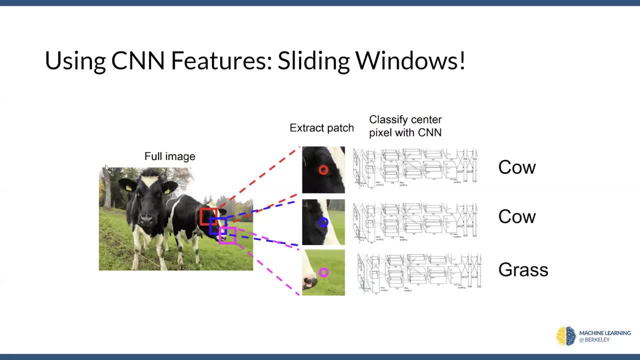 Right. So we're sliding across And you know, maybe this pixel is saying sky. This pixel is saying tree. This pixel is saying tree. This pixel is saying tree. This pixel is saying cow. This pixel is saying cow. 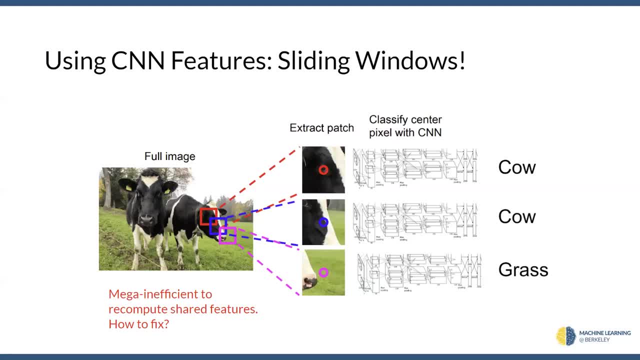 Things like that. This is as we saw last time. sliding window approaches in general is just very inefficient, Right. It's like once again, we're, you know, recomputing bait. shared features, Right, We're kind of, you know, running classification over the same area lots of times. 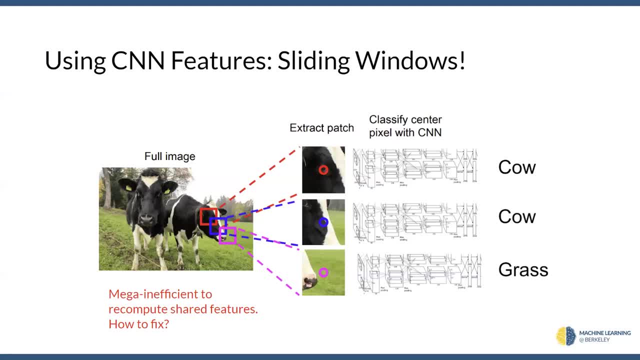 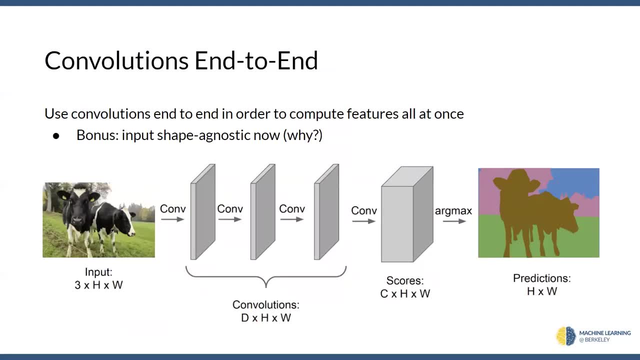 So how do we fix this Right? Well, we talked with this again on Tuesday, But this is kind of a different approach to it, So we can do convolutions end-to-end again, Right- convolutional network, instead of running it multiple times. 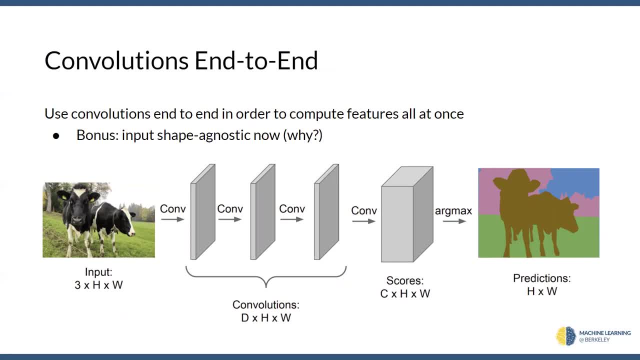 we can just have one sort of convolutional operation that we can run over the image that, ideally, will perform all of the desired effects that we want without having to do the sliding window approach. So, in this case, what we essentially have, so OK. 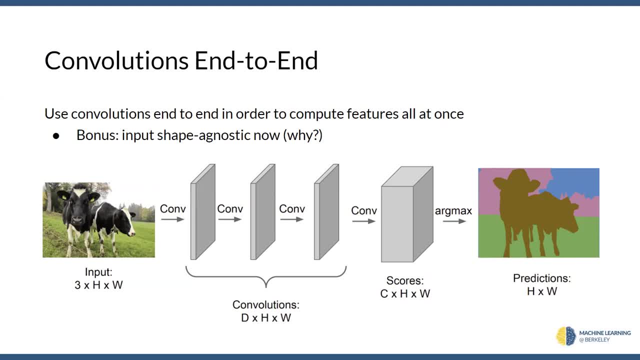 to clarify. there's one kind of caveat to this situation, which is that last lecture we were talking about classification, like detection, that kind of thing, And so our output was a defined size in the sense that when we're talking about the case of classification, 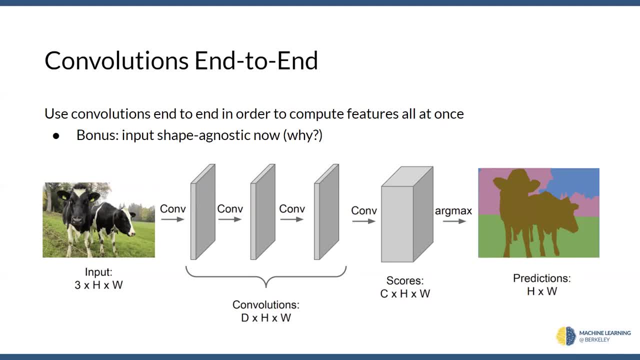 with localization, our output was going to be one classification, one x and y-coordinate pair and one width and height pair for the value box, Whereas theoretically, with segmentation, we want our output to be the same size of the input and essentially contain in every single pixel. 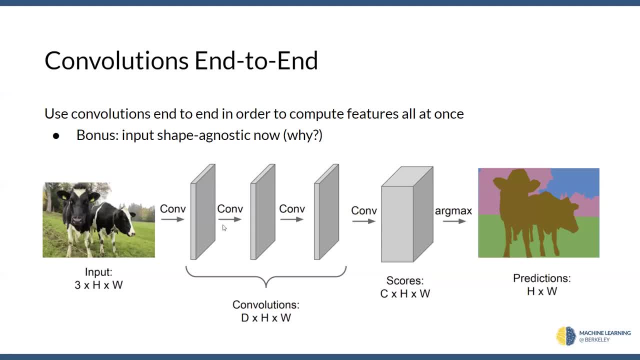 tell us what that object is Right. So one kind of bonus of this end-to-end convolutional approach is that the whole system is size agnostic of the input, And so it's maybe a little bit confusing. It's like, well, if we're plugging the image, 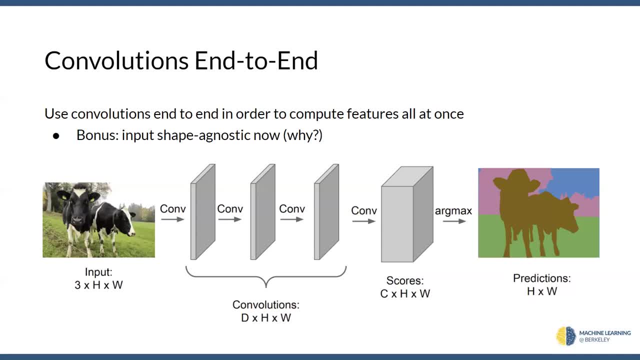 into the convolutional neural network. how is it sized? Isn't it expecting a certain number of inputs, that kind of thing? But essentially the way that you can think about it is that if our convolutional layer is that you can use that kind of filter explanation where 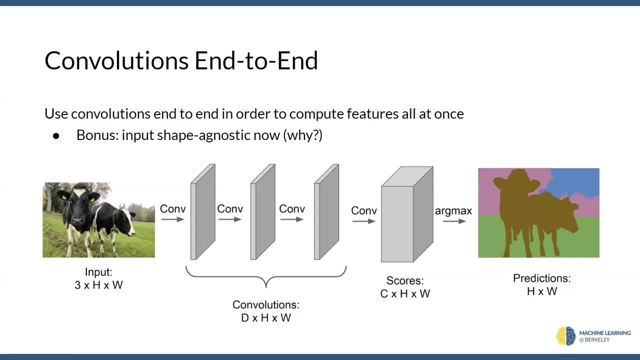 we have a convolutional kernel or a filter that's kind of running along the image and then it just goes on by the step size moving over each time. If we just take that filter and keep running it, there's no required size. 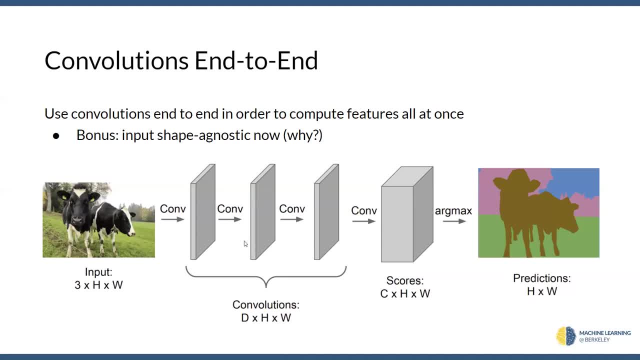 We're not decreasing the size of the network using pooling layers or anything like that. We're literally just running the convolutional network over getting an output layer. that's exactly the same. You notice this is a three-channel. If we look at the actual numbers, this input image. 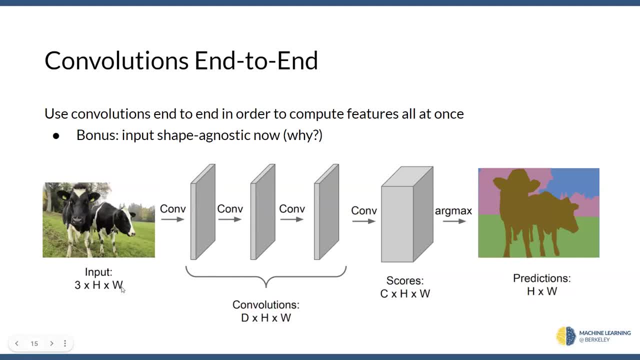 is three channels, like the red, blue, green channel, and then a width and a height. When we run our convolutional layer over, we're still getting a width by height, length, volume. It might have more depth or less depth, depending 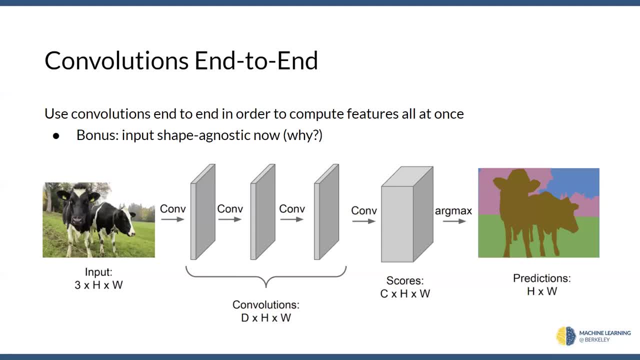 on how many channels we have internally. But the basic idea is we're just passing that convolutional filter over, so we don't have to worry about the size changing or that kind of thing. We can just kind of run everything over And the predicted output will map one-to-one exactly. 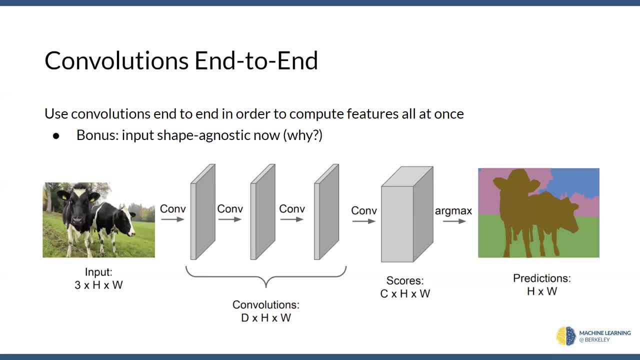 with the original image. Yes, Yeah, great question. So, yes, theoretically, there's a couple of different ways that we can do this. So, first of all, if we have like, let me get some chalk. So, for example- let's just take a very trivial example- 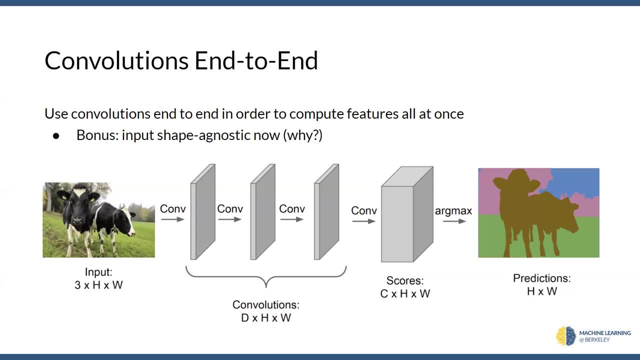 where we have a two-by-two image Right And let's say, our filter is three-by-three Right. So one thing that we could do is we could essentially use padding Right. So the idea is, if we just like, padding is complicated. 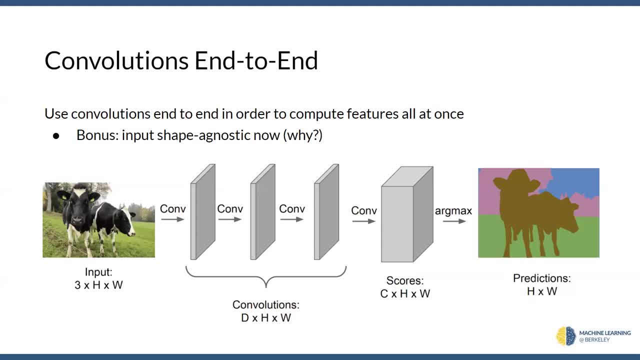 and shouldn't necessarily just do this, But let's just say we add zeros to the outside, like all the missing pixels in the image. Right Now, when we run our three-by-three filter over, right, it's going to run here. 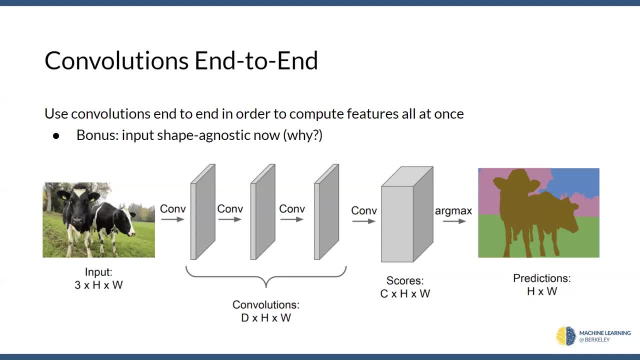 It's going to output that into the first pixel Right And then when we shift it over one, it's again using up those padding bits right to classify this one and then to run on this one It's going to move into there. 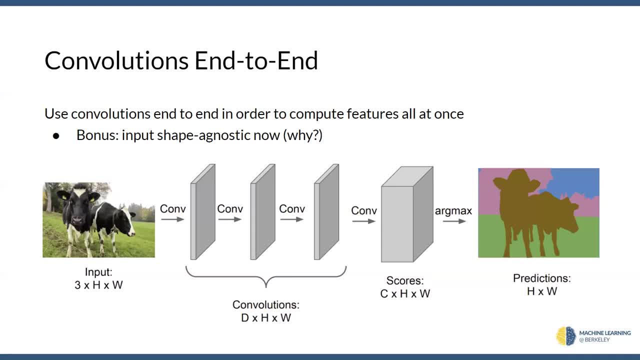 Right, And the idea is, if we have stride one, we have enough padding, right. It's like we're not going to be. we don't have to be decreasing that size, And I guess just a quick aside. but when doing padding and that kind of thing, there's a lot of different. 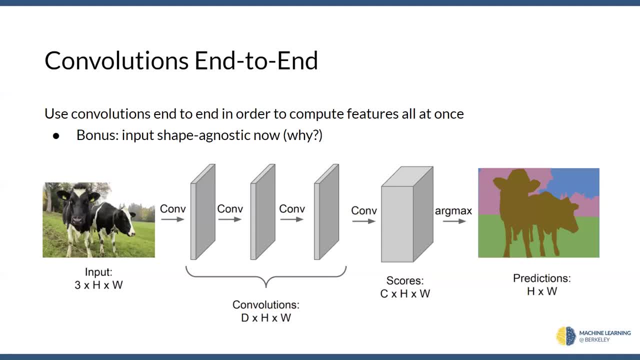 I don't know if we've talked about this yet, But padding with zeros is kind of weird, because then it's essentially you're treating the network is seeing as if there's a black wall at the edge of the image. There's a bunch of different kind of approaches to fix this. 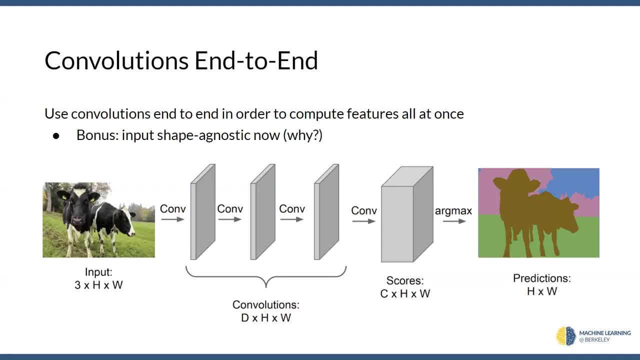 Yeah, one second. One of the things you can do is you can kind of mirror the edges. So, for example, we can take these pixels and duplicate them here. Or, even better, you could take this whole thing and then flip it over and kind of duplicate. 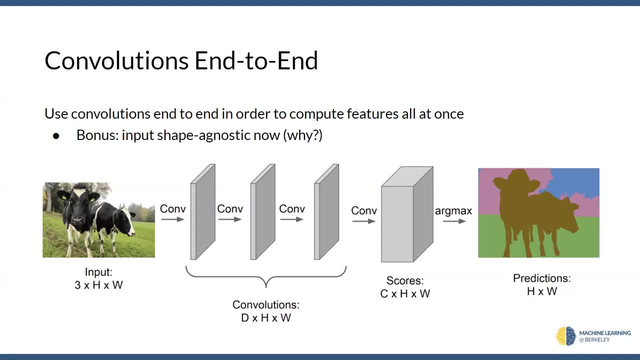 so the padding kind of matches the colors on the inside. But yeah, great question. You had a question. Yes, I'm not sure where your slide is. Take an art next, Or do you take an art next layer? How does that? 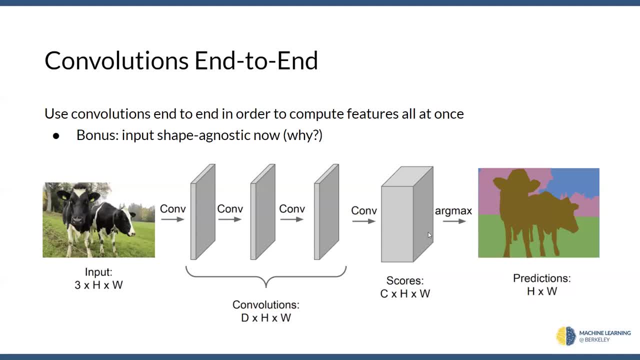 I think it's like the final thing. Yeah, so the basic idea here. OK, really, you can kind of just think of it as essentially, as we kind of go through these convolutional layers right, And then as we kind of get to the final output. 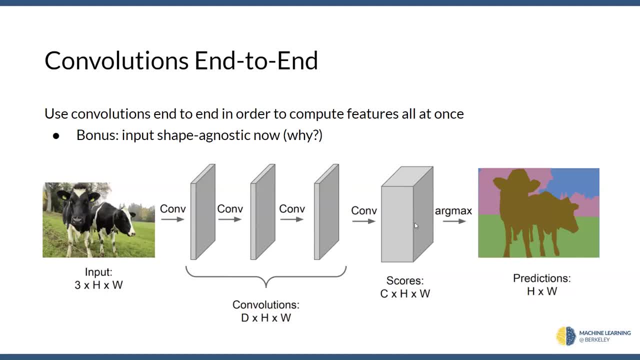 the final output is going to be a volume that has size, width by height of the image And then the depth of it is. essentially, each slot in the depth is talking about a certain classification output. So the idea is we're essentially finding the maximum classification. 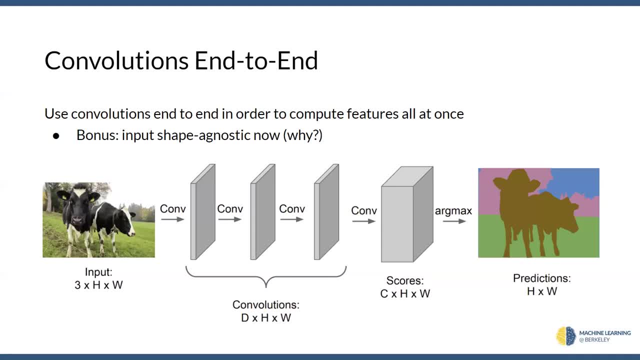 output for each pixel. So that's like the number of classes, right? Yeah, exactly, C would be the number of classes, That would be it, And so in semantic simulation that's sort of the prior right. It's a bit more. 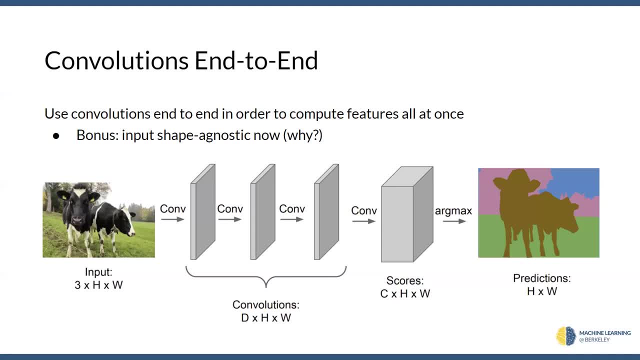 Yeah, It's a bit more of a background or some. So, yeah, I mean there's lots of different. like we talked about this a little bit last time, There's different ways to kind of encode things, But for right now, just think of it as it's like a one-hot encoding. 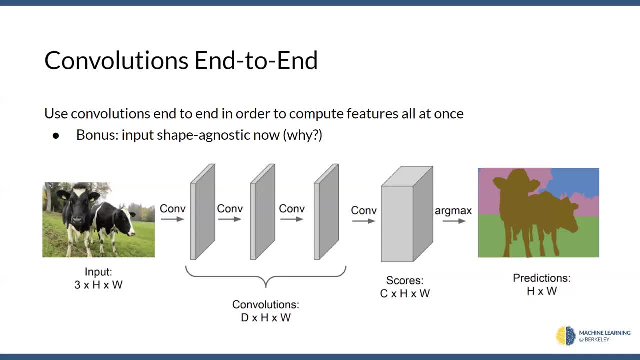 where each class maybe there's a one, if it's sky, There's a one in the next, but if it's like a cow or et cetera. Does that answer your question? All right, great, Yeah, so oh yeah. 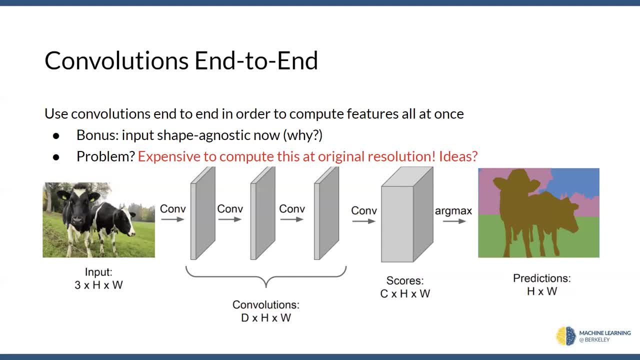 OK, So the problem with this is that it's pretty expensive to compute this at the original image resolution. And what do I mean by that? Well, I mean, let's say you have like a 4K image, right, And it's like maybe you have- I don't know- 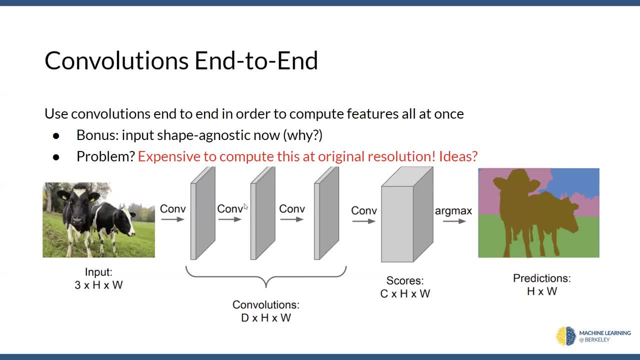 like 20 convolutional networks or something right. I'm just coming up with random numbers, right, But it's like the idea is we're still doing that, excuse me, we're still sliding that filter over and doing that kind of computation on like every single pixel. 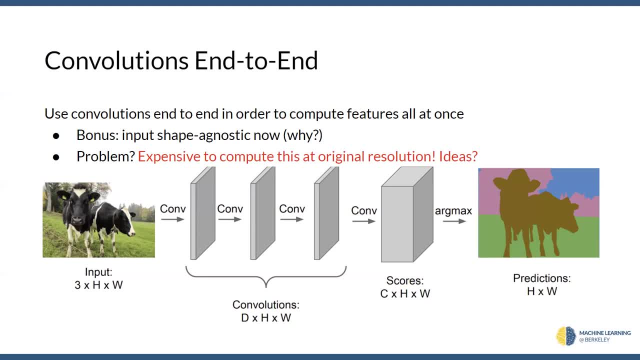 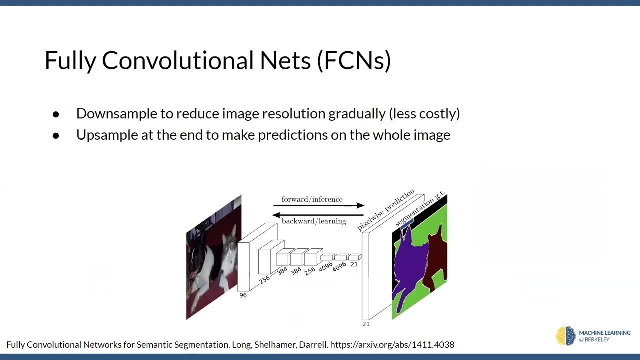 Right, We're still doing quite a bit of work right, And so as long as we kind of maintain that original resolution, it's going to be kind of hard to shrink that down. So one potential solution to this is to essentially downsample. 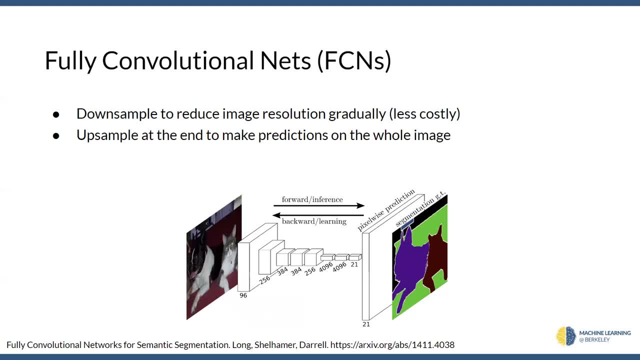 the image gradually and then upsample it at the end. So what do I mean by that? Well, essentially, what we can think of is: if we look at this image here, right, It's like we have this input image, right. 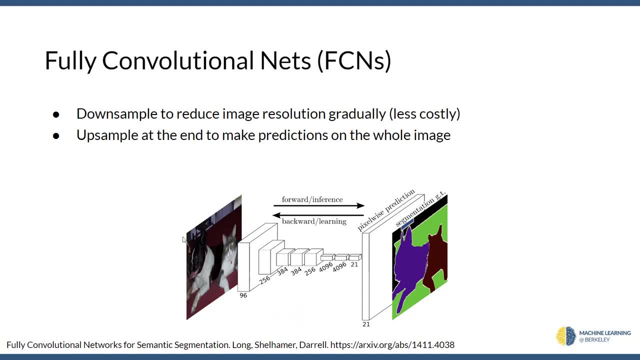 And then when we run our first convolutional layer right, We can, instead of doing this like padding thing, where we want it to be the exact same size, and having like a stride one or that kind of thing, we can maybe up the stride a little bit. 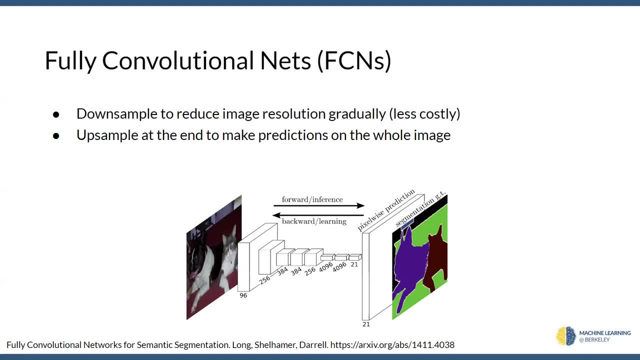 get rid of a little bit of padding right. Do something like that So that the output of running the convolutions over once is going to be smaller than the original input image, at least smaller in width and height. maybe it's a little deeper. 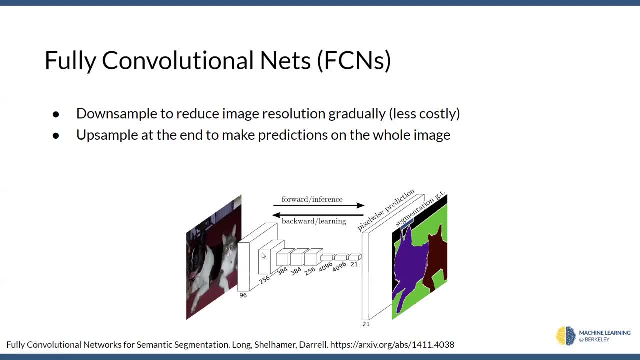 something right. But the idea is we're kind of shrinking it down And each time we're kind of shrinking the image down further and further, all the way down to like this example: It's like I don't know, it's 21 or something. 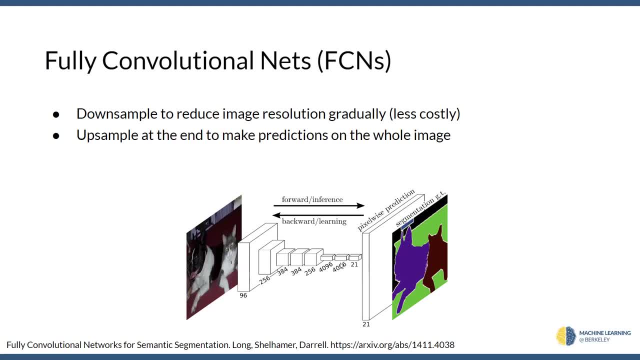 I don't actually remember what these numbers are, But the point is right. It's like the volume that we're outputting is getting smaller each time, So we're essentially downsampling the image every single time, right? You can think of it as we're taking the image, right? 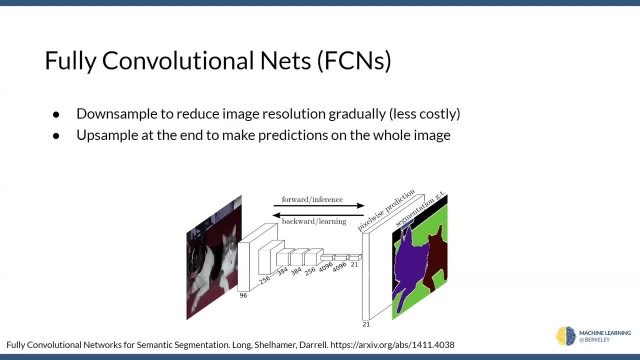 The convolutional neural network, ideally, is going to be like extracting information, removing redundancy from the image as it kind of passes over And each level is getting more and more abstract. in the sense of ideally, maybe it would be collecting the first pass. 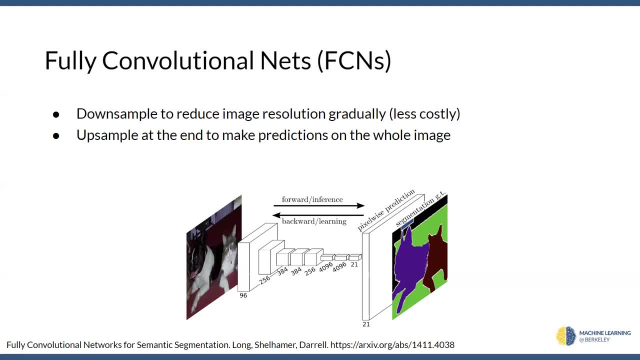 would be collecting information on edges or that kind of thing, And then the second pass would be combining those different features to maybe get more high-level understanding of the image or something like that. right, It's all just theorizing, But the whole point is that we're kind of downsampling this. 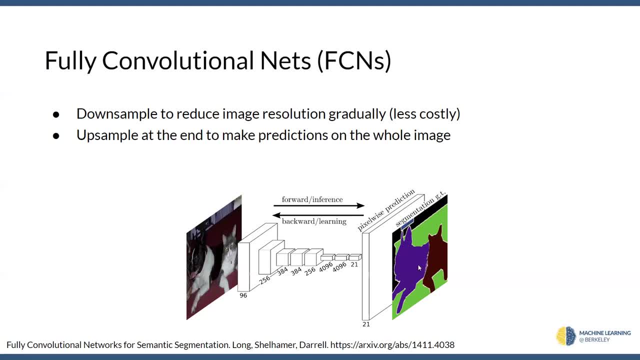 We're getting down to a much smaller kind of volume at the end. But then of course we have this problem that we want our output, our segmentation output, to be the same size as the input image. right, Because we don't want to output if we input a 4K image. 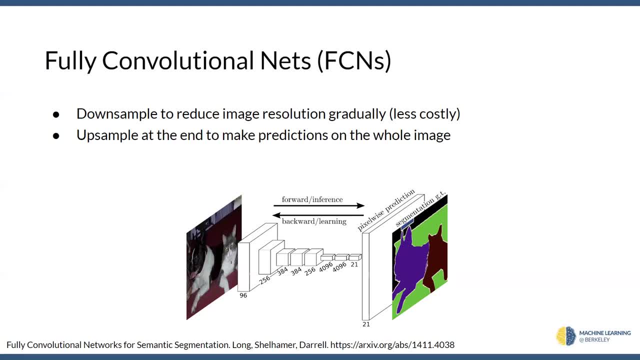 we don't want to output a two-pixel by two-pixel segmentation map, right? Because that's not going to be very useful if the pixels don't really match. So we somehow need a way to kind of take this small volume and somehow transform that small volume back into an image. 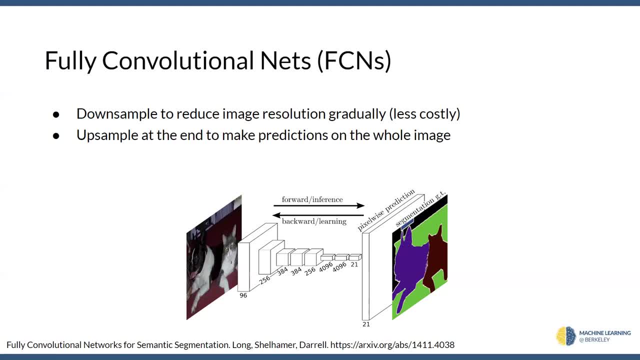 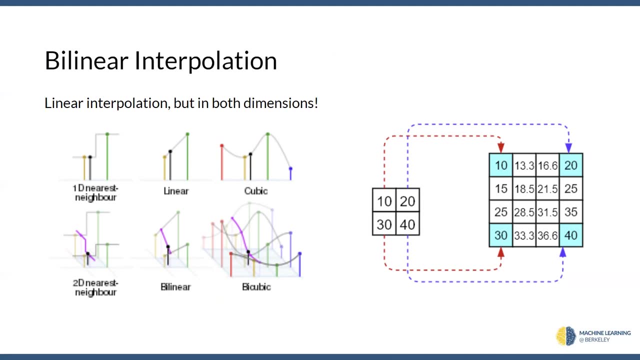 the size of the full image right, Which is a little weird, right, Like, how do we do that? So there's, yeah, how do we upset? So there's a couple ways to do this, The classical approach that I'm sure if you guys have ever used Photoshop, 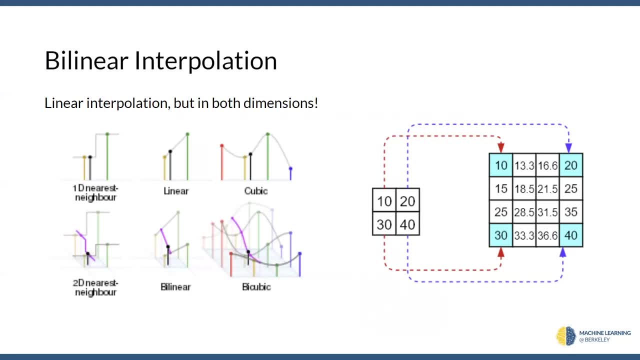 or done anything with that in the past. you guys have definitely seen this before, where I don't know if you guys ever used MS Paint. but if you put an image in MS Paint and you scale it up a little bit, it gets all pixelated and gross. 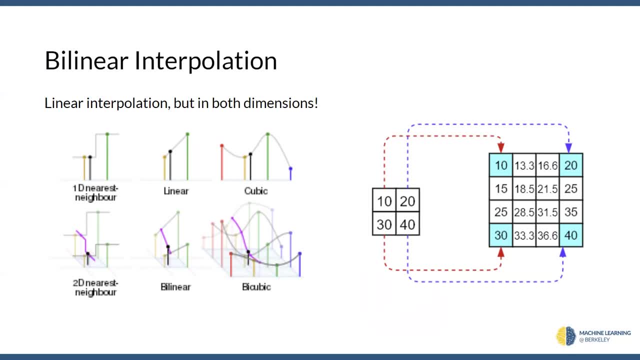 because MS Paint is, I'm pretty sure, by default using nearest neighbor, or at least maybe it used to, which is disgusting. But essentially the basic idea is, when you scale up an image, you can essentially think of it as we're stretching the pixels out. 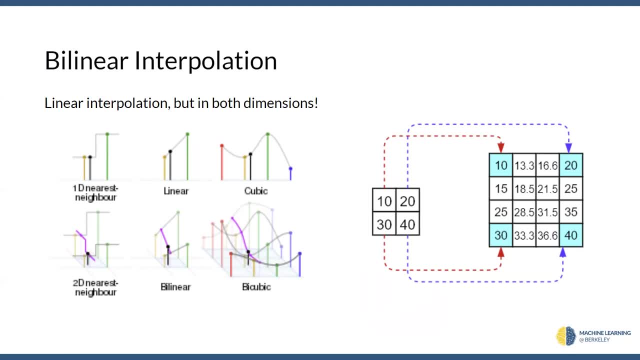 and then now there's kind of new spaces for new pixels to be formed, And so an interpolation function is essentially deciding what those new pixels should be right, How to kind of blend between the two pixels we had already that are now separate enough that there's a new one that's needed in between. 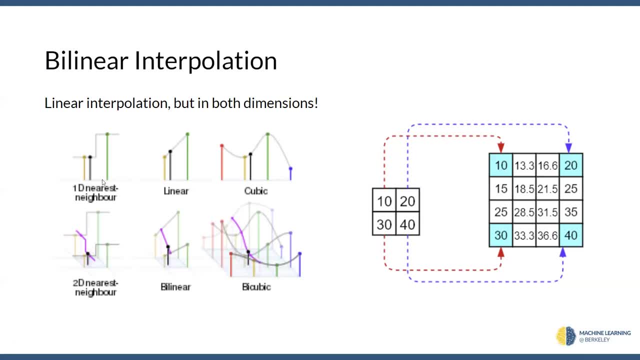 So nearest neighbor is one that I was making fun of. Essentially, the basic idea is that we're literally just taking the value of the pixel it's most adjacent to. So if we have a small tiny image and we scale it up really large, 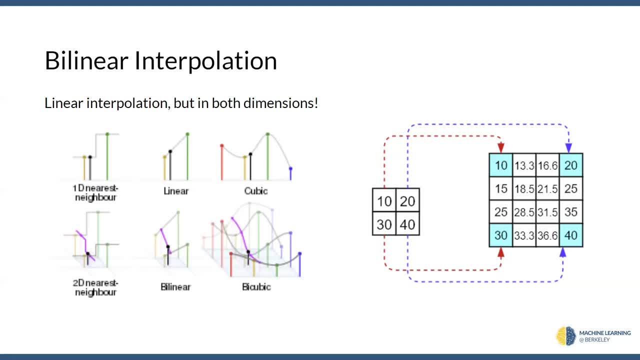 we're just going to get giant pixels because we're not doing any sort of blending, We're literally just selecting the nearest pixel. You can do some sort of a linear interpolation, where it's like you take the two edge pixels and you find the color that's halfway. 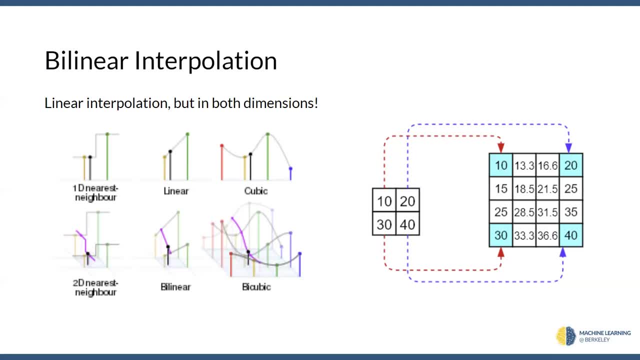 in between them, right, And it's like you can do something like that, The option that most software that can use Photoshop and you try to scale up an image. I believe the default is going to be either bilinear or bicubic interpolation. 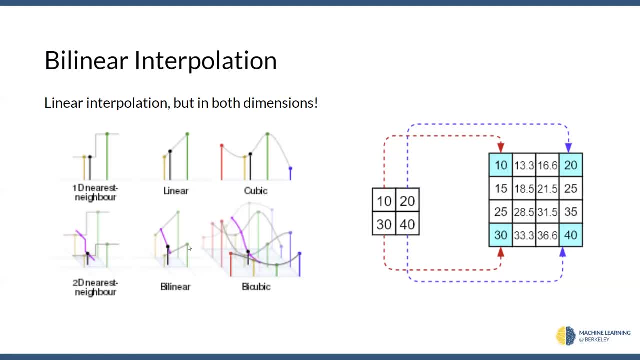 But essentially the idea is that it's essentially taking the color information from both the pixels to the side and also the pixels up and down, and essentially computing some sort of linear average between those to find the output color. And so the idea is that if we take this image on the right, 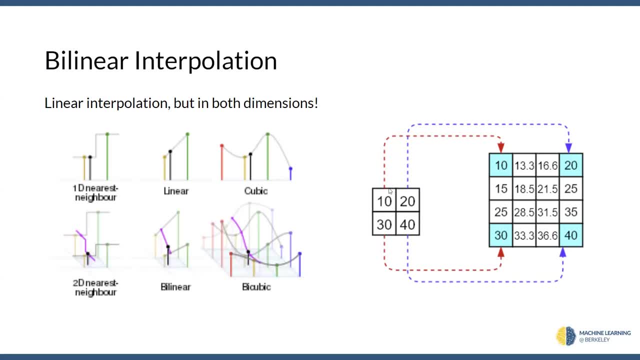 and it's like we want to stretch it out to four times the size. we can put those pixels on the corners and then we can use bilinear interpolation to kind of fill in the missing spots, And this theoretically works. It's not a wrong approach. 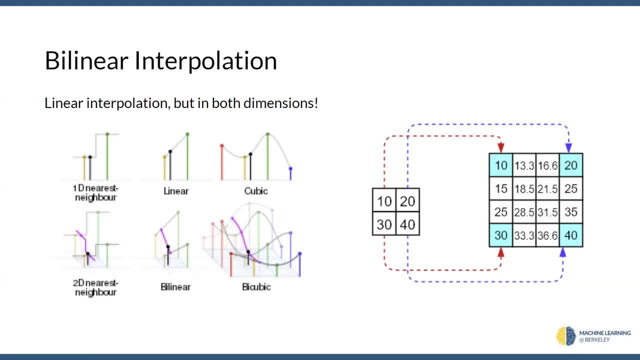 But the issue with this is that what we're really doing is essentially scaling up the image and then blurring it a little bit, as opposed to filling in detail that we're missing, right, And so a way that we can improve this is by, once again, 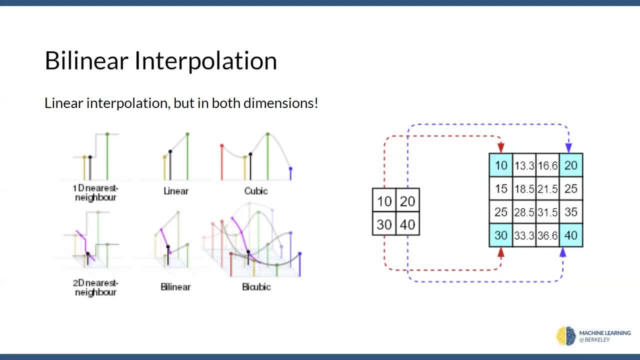 we can move from a classical algorithm to a learned algorithm, right? So the idea is we want to upsample, But instead of upsampling with bilinear relation or something like that, we want to have some sort of neural algorithm or something that can learn how to upsample images, right? 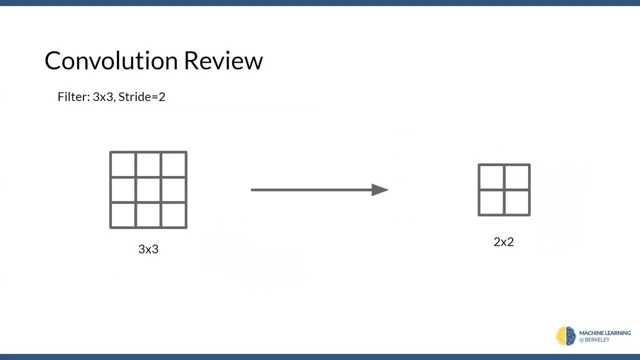 So I already kind of went over this, but I want to do a quick review of convolutions because I'm about to introduce something called the deconvolution, which is pretty easy to understand if you understand convolutions. So I guess just very briefly I can go over again. 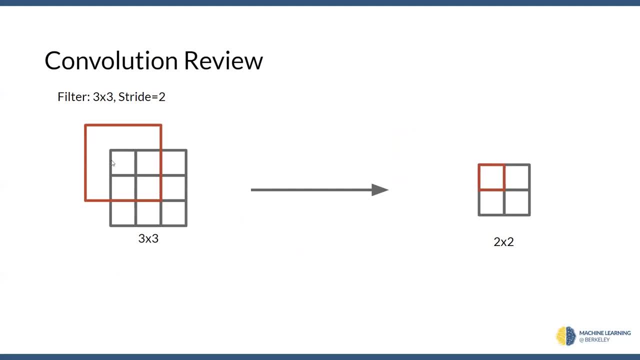 It's like you have a filter that you're kind of passing over- like in this case 3x3. And you're essentially taking all of those values and then you're multiplying them by the weights of the filter and then kind of summing those all up and putting it. 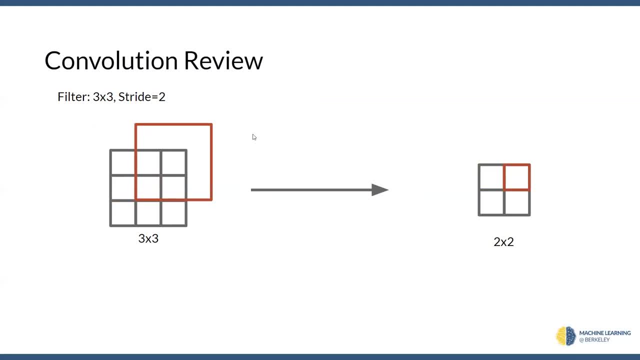 in the corresponding output pixel right, And then you shift over by the stride each time and you kind of keep passing them on And you kind of go through that until you've gone through the entire thing. So the other thing you can kind of think of. 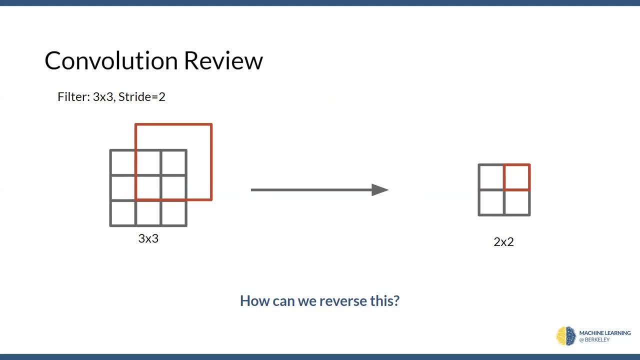 is how can we kind of reverse this process, right, Like we want to take essentially the same like a kernel, idea of a kernel, like kind of passing over an image, right, But instead of passing over some sort of input layer and then getting a small output layer? 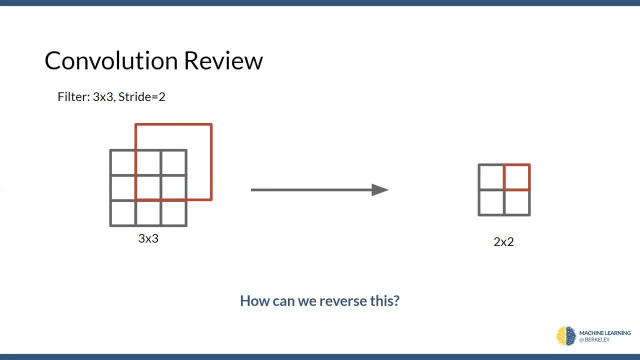 we kind of want to take this and do the opposite. right, We want to pass over a small input layer and somehow project that through some sort of filter Right Onto a larger output. right, So to that enter the deconvolution. 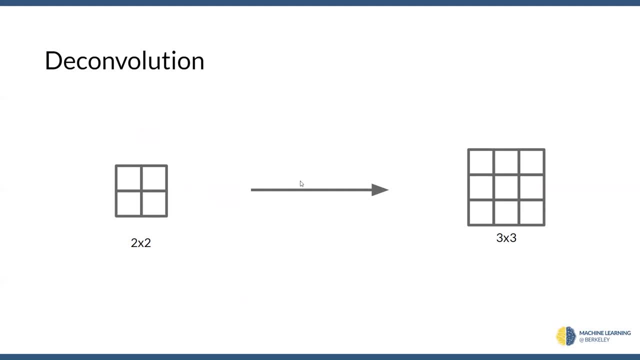 So it's literally I just flipped the diagram right. We have the smaller one on the left and then the larger one on the right, And so the basic idea is we are literally- like you can kind of think of it as we're literally flipping- 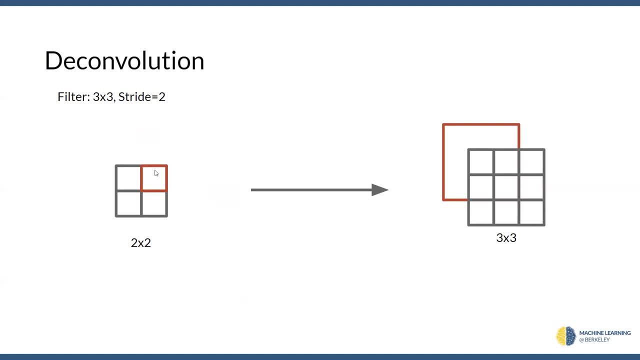 the diagram that we had before, And I'll get into how that actually works in a second. But so, instead of passing the filter over the input layer, you can think of it as we're passing the layer over the output And then we're moving pixel by pixel on the input right. 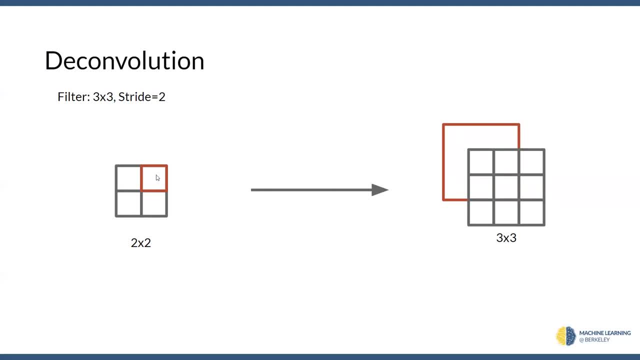 So actually I have some slides here, But honestly I think it's going to be a little easier if I just draw it. So I'm just going to draw an example. Let's say we have one or that's not a one. 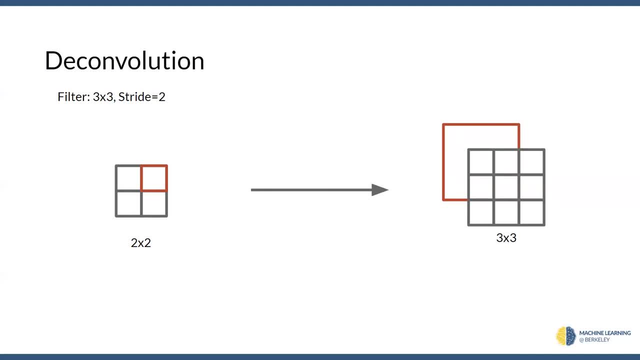 I can write down this All right: one, two, three. Also is my handwriting way too small. Can you guys see I'm good, Perfect, OK, one, two, three, four. Let's just say we have this. 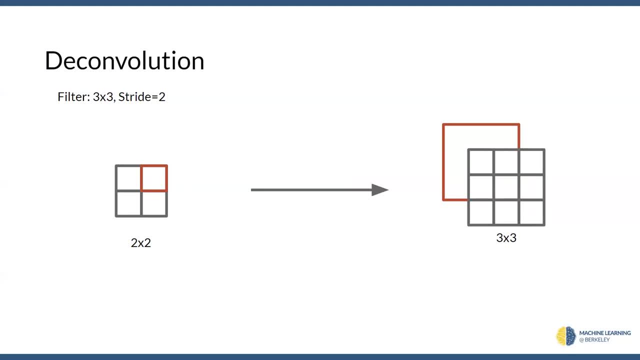 This is very simple input image right, And we want to upscale it to like a three by three right. So what I said before is we can start, let's say: then let's also say we have like a three by three kernel right. 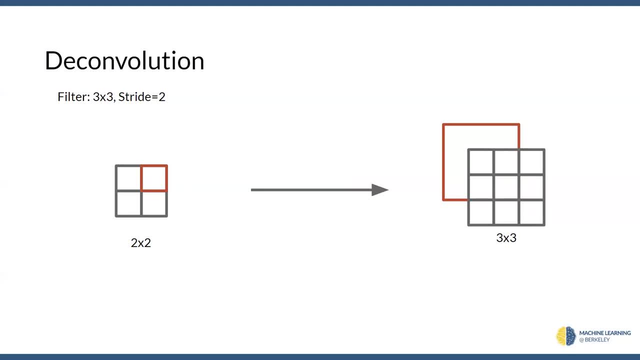 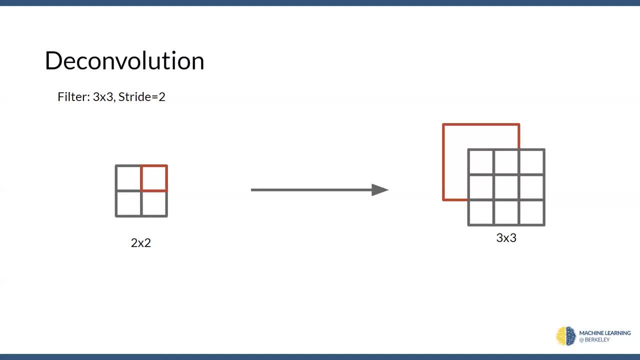 We're going to look at the first pixel of the first image, right, And then what we're going to do is we're going to take our filter and we're going to place our filter over the output layer centered around this pixel. OK, 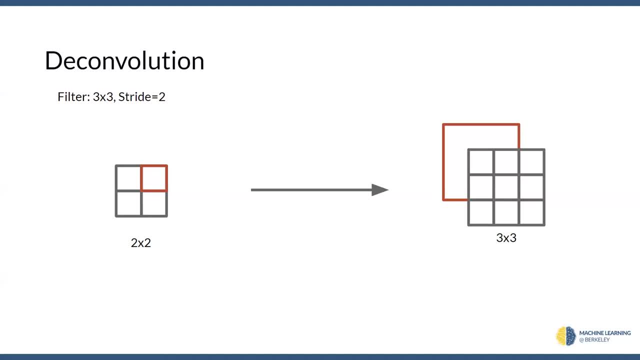 And essentially what we're going to do here is we're going to take this input value and we're going to multiply it, And then by each of the output values in the output, or, sorry, by each of the filter values, and we're going to essentially project that or kind of imprint. 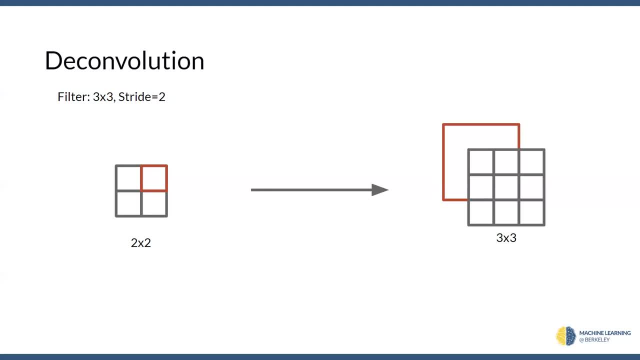 that onto the output, right? So in this case, like if this box were placed over, like this whole section is just like outside of the range. so I don't have to worry about that, right. But you can kind of think of it as it would be, maybe like one. 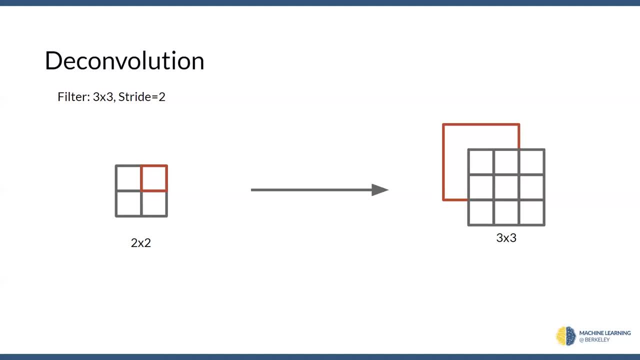 one times one right, That's going to go there. One times zero, that's going to go there right, Like that: One times zero and then one times one right. So on the very first pass we've kind of added: 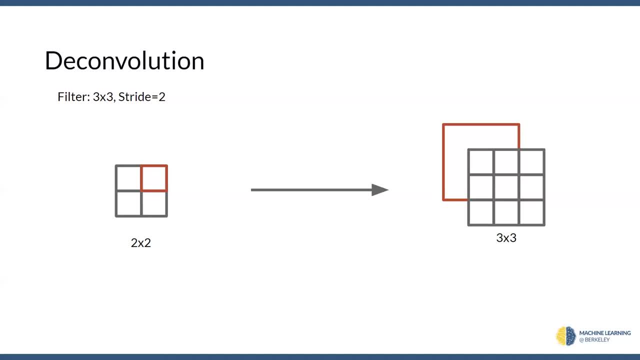 And again, this is just this number multiplied by this and then placed on the corresponding slot on the output right. And so we can do that once and we get some values kind of magically appear here right, And then all we have to do is we can shift over to the next pixel, right. 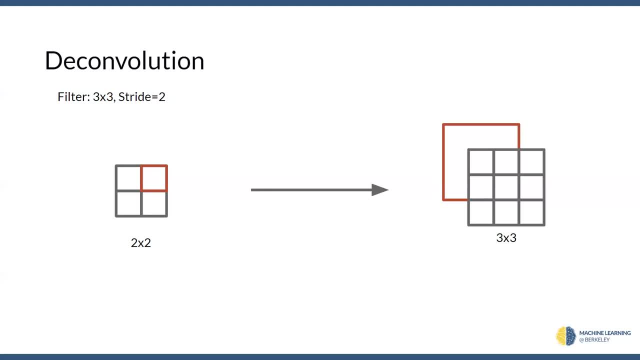 And now what we can do is we can maybe shift this box over as well, Right? So maybe now this filter is now looking at this region centered here, right? And we can say, okay, let's take two, two times two is, or two times one is two, right? 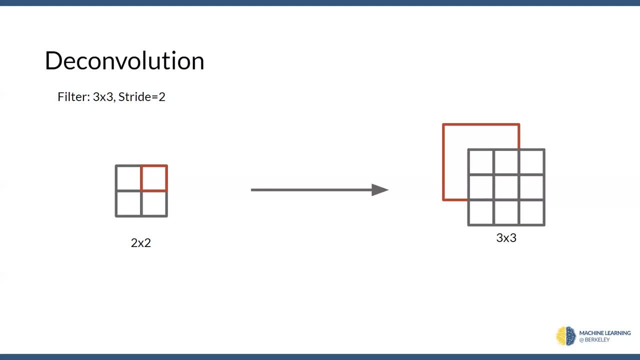 This is not two right. We can say: you know, two times zero is zero right, Two times one is two right, Et cetera. The point is you can keep doing this right, But you may see a problem with this, which is that we're going to end up like overriding. 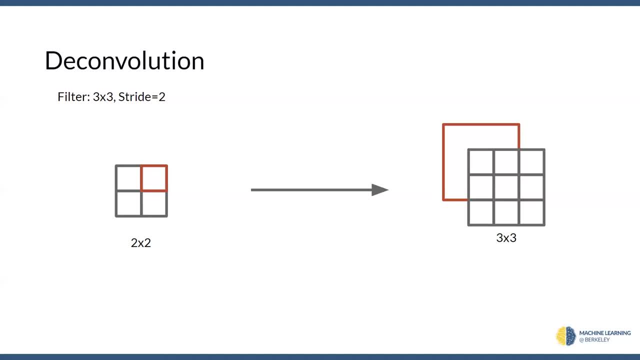 values that we're doing And it's like kind of weird, like what's the point of this right? Well, the idea is that if we would add a value to a node that's already has a value, we just add them right. 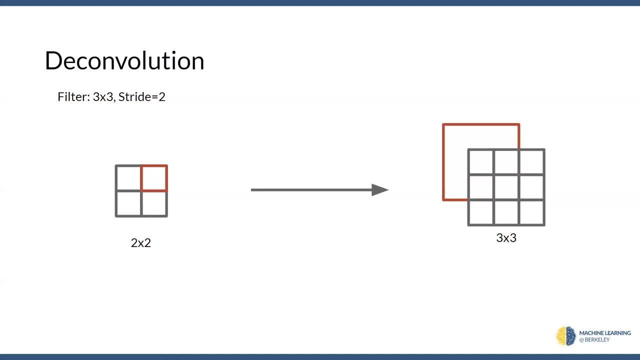 So the idea is is that these output values are essentially going to become like a sum of the kind of projection of the input values through the filter crest onto that image, right? So I'll go over it kind of again, cause it's a little bit weird, but you can kind of think. 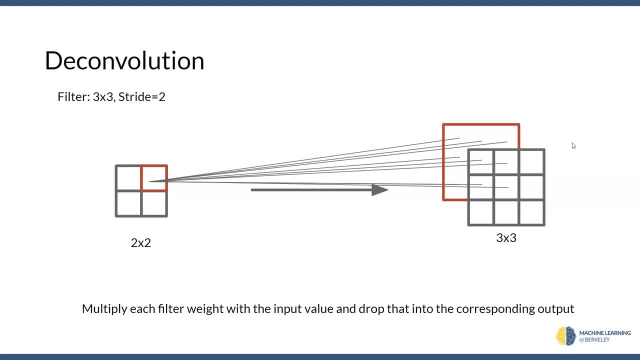 of it. as you know, it's like we have this input pixel. we multiply each weight in the filter by this input pixel and then kind of think about it as like we're pressing that down onto the output image And that there's already a value there. 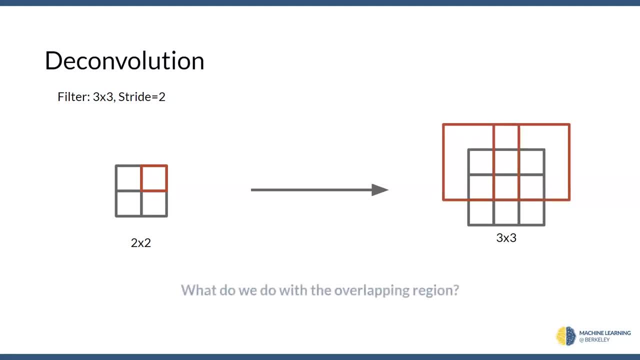 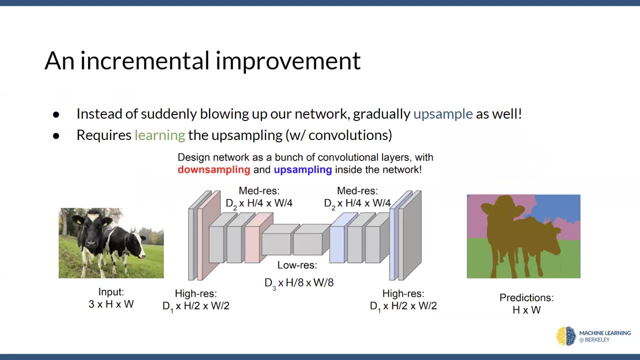 We just sum it up Right And again we can keep shifting that over: Yeah, And so that's a, that's an accomplished. So using this, we can do something a little cooler, which is that we can take like, essentially: 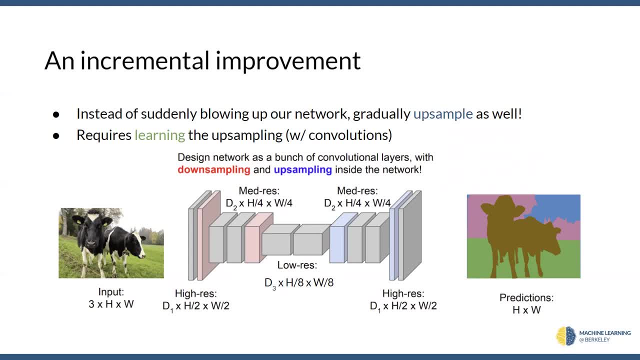 an incremental approach to the problem, right Where We can, you know, start with this really large image and then we can run the convolutionals, convolutions over it to downsample it into some, you know, low res internal representation with maybe some depth, but it's, like you know, pretty small. 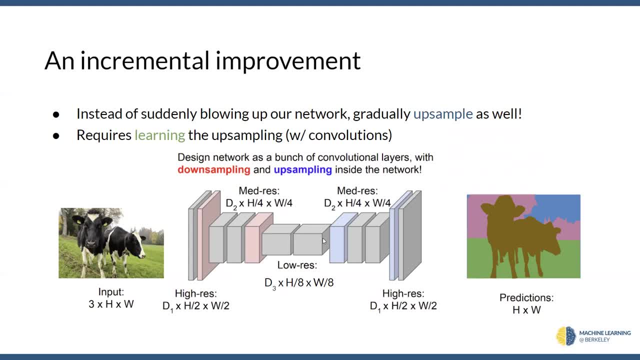 And then what we can do is we can use D convolutions to start raising the size back up right To slowly offset, And I guess there's two benefits of this approach as opposed to the approach that we talked about previously. So, first of all, the big one is that 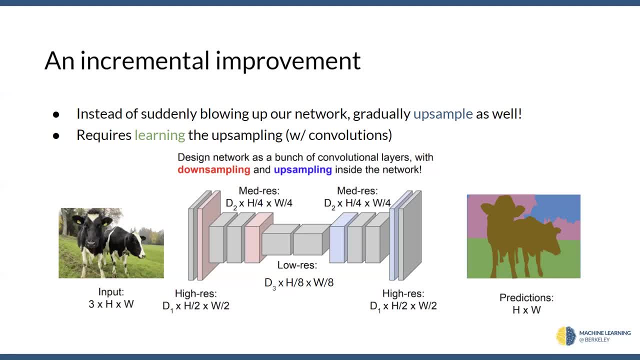 The upsampling is learned. It's not just a classical algorithm, right? It's something that can learn and can adapt to the problem that we give it, which means that, instead of just like filling in, you know the blend of the pixels with like what. 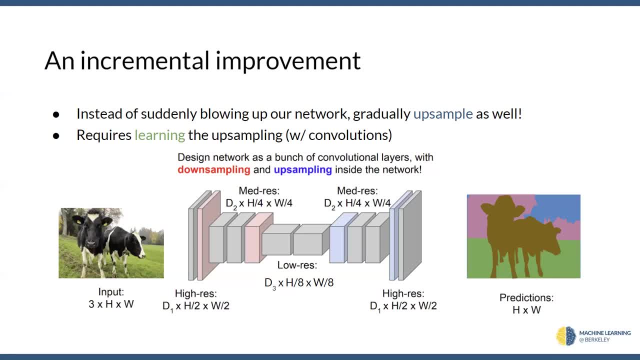 they like average color value is right. It's like, theoretically, the D sampling could kind of learn to, you know, maybe like fill in certain edges or like knows a certain shape, And so when upsampling it might refine that shape a little bit right. 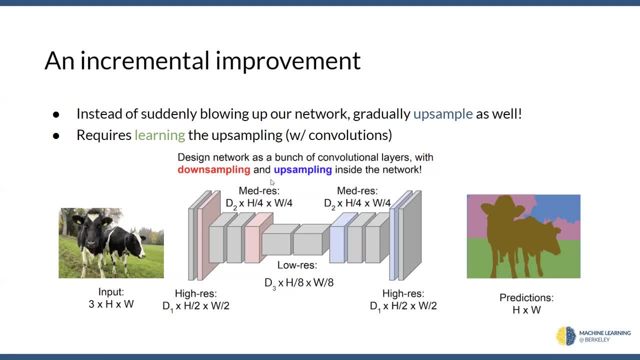 It could do you know, different cool kind of approaches like that, Yeah. And secondly, the reason that we're doing this upsampling like slowly instead of just doing it in like one giant push is, is essentially just that we get, like you know, more chance. 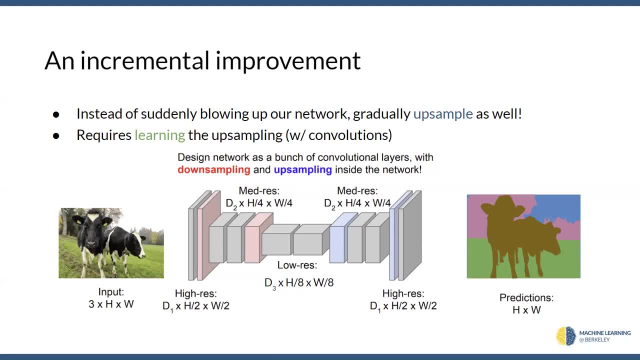 for you know, if we, if you think about like doing this D convolution process right, It's like there's more intersection between things, There's more opportunity for overlap If we kind of do that over multiple passes. Yes, 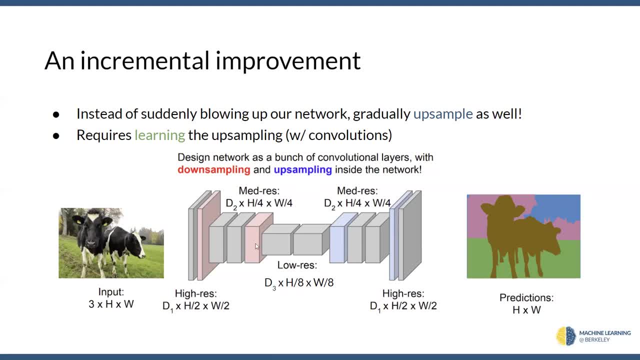 So the first half of the network, are you still using the soft level of like a max or something down to this? Yeah, Yes. So So the D convolution itself is: does offset Right, Because I mean, like in the example that we just showed, right? 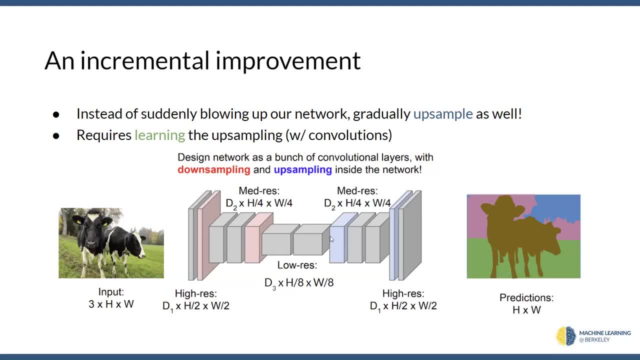 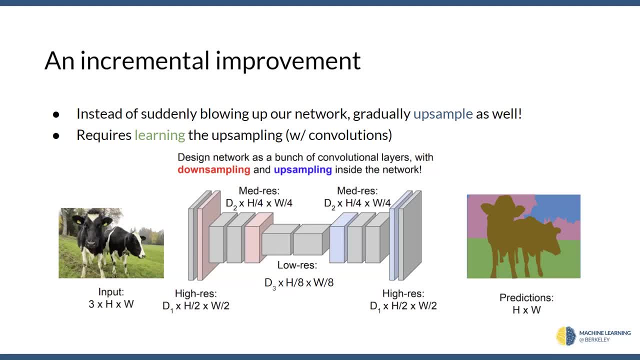 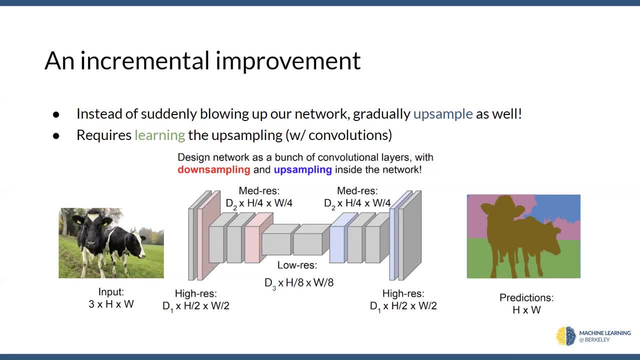 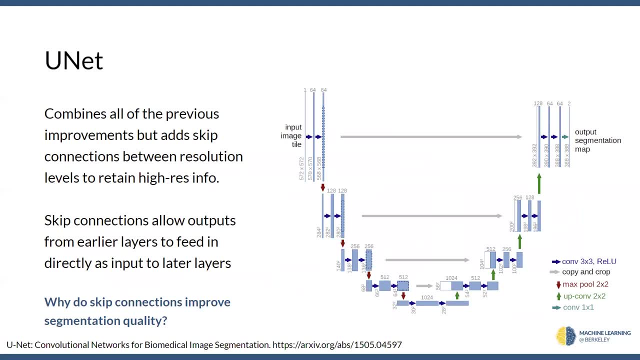 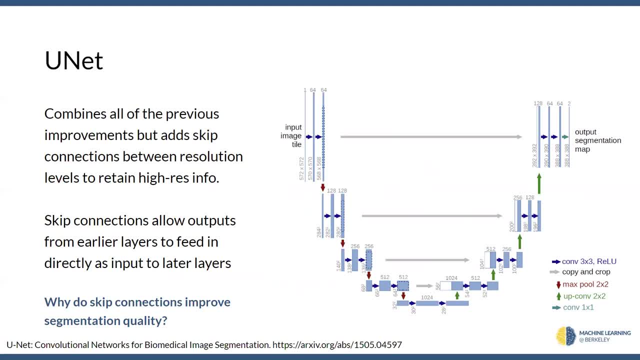 Okay, Yeah, So if we take this approach and add in a couple little bells and whistles, which we'll get into in a second, we get something called you know So. So kind of previous improvements that we talked about, with the addition of one little fancy. 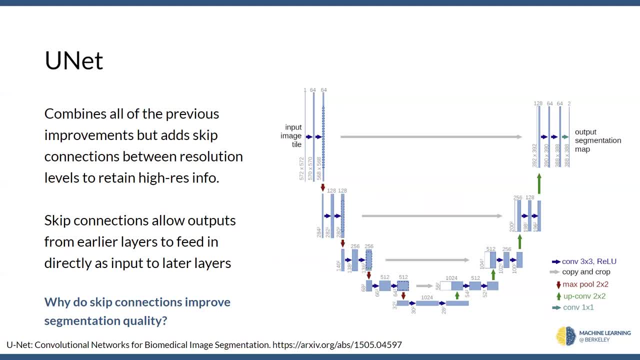 feature which is skip connections. So I don't think I don't know if we've talked about those. we have. Great, Okay, I have to explain it. So current skip connections idea, right, The whole idea is that you know it's like it can pull in, you know information from you know less. 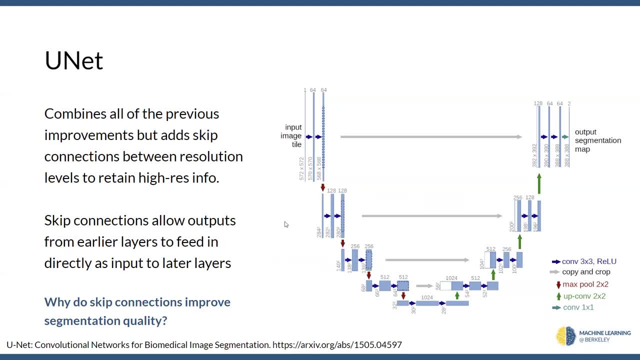 processed parts of the process up all the way till the very end, Right. And so you can see, right, we have this image as we kind of pass through. we're slowly like downsampling it until we get to this internal state and then we start upsampling. But when we're doing the upsampling, 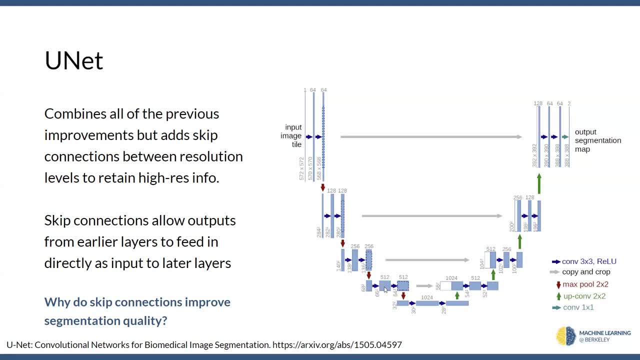 we pull in information from the corresponding level of the downsampling path. So the idea is like you know, for example, in the very last section of the network, right, it's like we're pulling in like potentially like detail information from the component over here, Right, Which is why 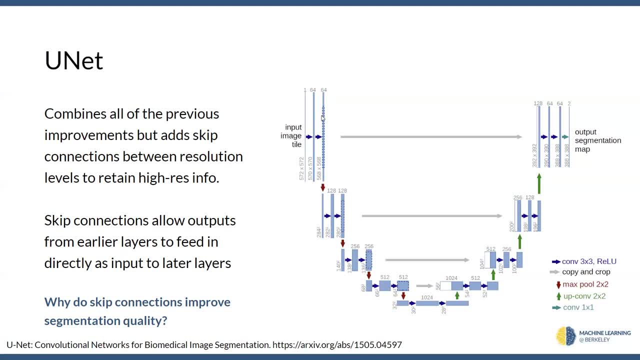 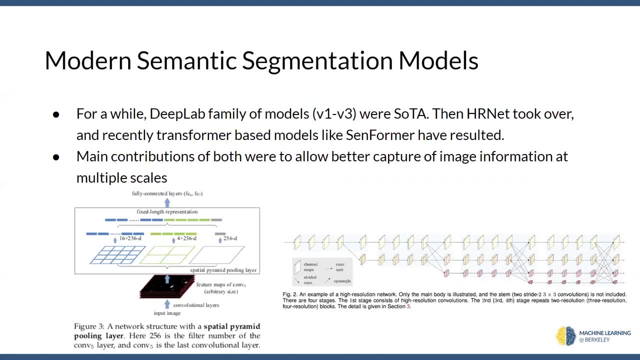 these skip connections are really, really powerful. They work really well for this type of task. Yeah So, Modern segmentation models, like it's essentially like there's a lot of continuations on kind of Unet, a lot of similar approaches. I can just you know. yeah, So for a while, family of models. 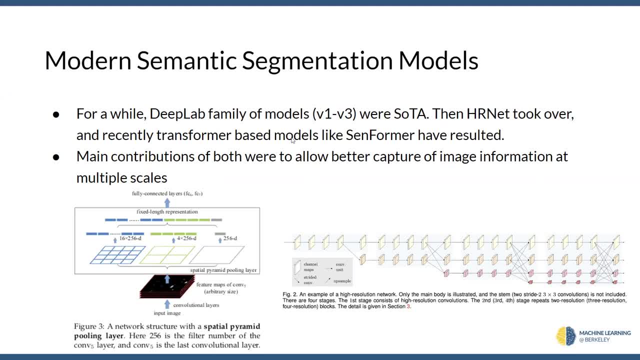 deep lab family of models which are the art nature ants took over and recently transformer based models like send former resulted. So the main kind of contributions of these were essentially just you know different methods to kind of better capture image information at like. 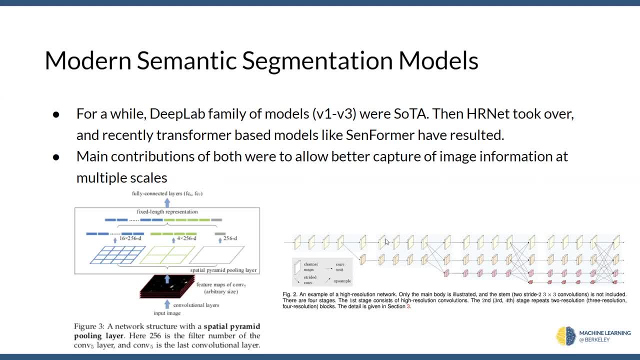 multiple scales. So like, if you guys want to look at these charts later, you can check them out. but essentially, just like you know different sets of connections and different kind of rates of down sampling and different kind of approaches like that. 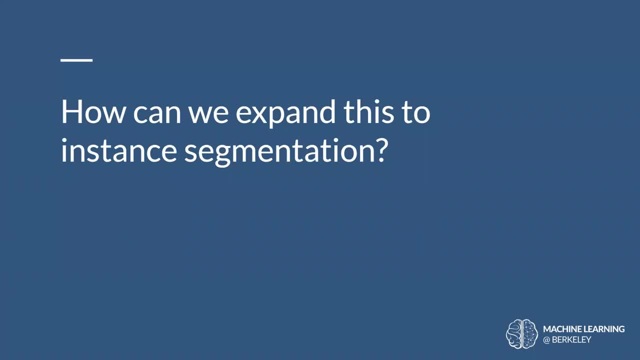 So all the things that we've been covering so far have been about like semantic segmentation. right, It's just classifying like this is cow right As opposed to this is a cow and then this is a different cow right. So how do we kind of expand this? 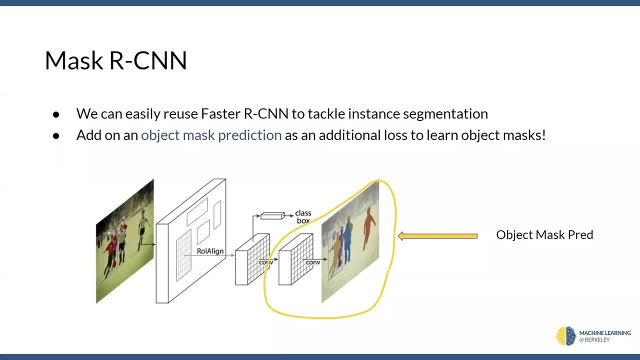 to instant segmentation. So one approach to this, we can go back to our old friend RCNN, We can expand it a little bit to just solve this problem for us. So if you guys remember RCNN, right Again, the basic idea is: 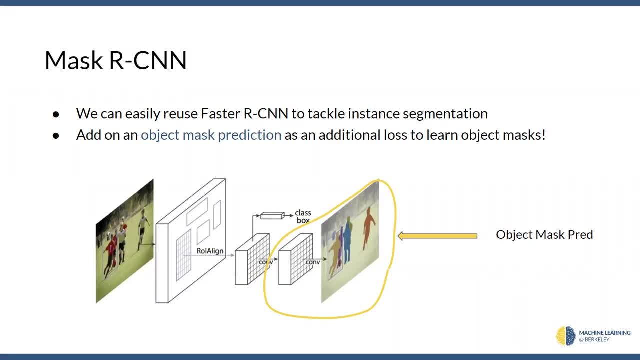 we use like a classical method to propose potential segments And then we, you know, essentially, like you know, find, like crop, the image to each of the segments and then run the classification on there And then if it matches, then we output that batting box and otherwise we 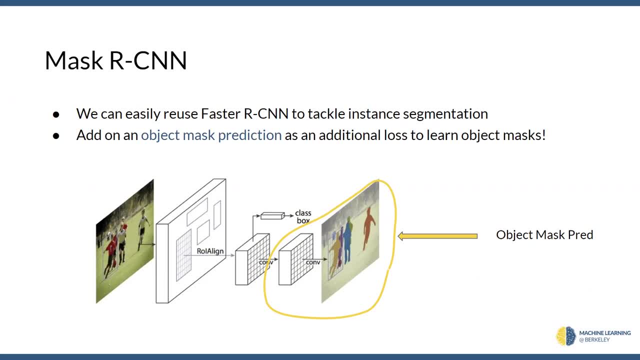 combine segments and then keep doing that over and over again. right, It's like I'm sure you guys remember this was a couple of days ago. But so essentially, mask RCNN is a continuation of that, where once we've kind of cropped that image down right, We classify it, but then we also add kind 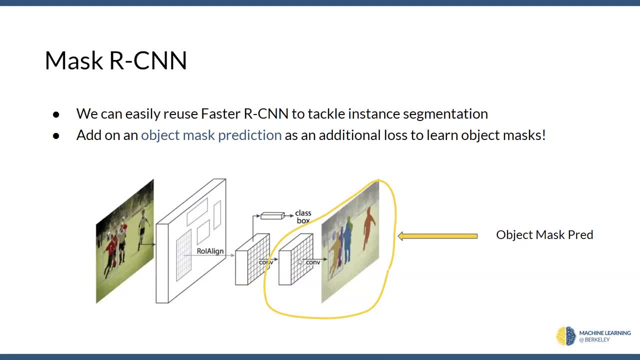 of an output mass prediction right Where essentially we run one of these methods right To essentially, you know, predict the location or run one of those segmentation methods to essentially identify that current object, right Within that kind of batting box. And so the idea. 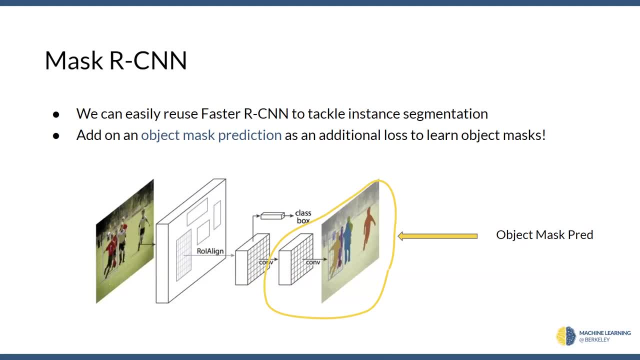 is if one batting box outputs you know like this shape or whatever, as like a person, right, And then a different batting box outputs you know this shape as a person, we can tell that even though they're both classified as people, they're different people because they represent. 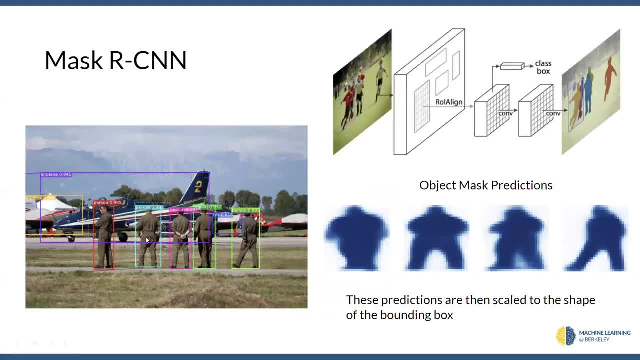 different objects, right? So yeah, you guys can see some examples of this, right? This is like some examples running, right. It's like able to kind of detect the different airplanes, able to detect all different people, And you can see these mass predictions that are coming out. 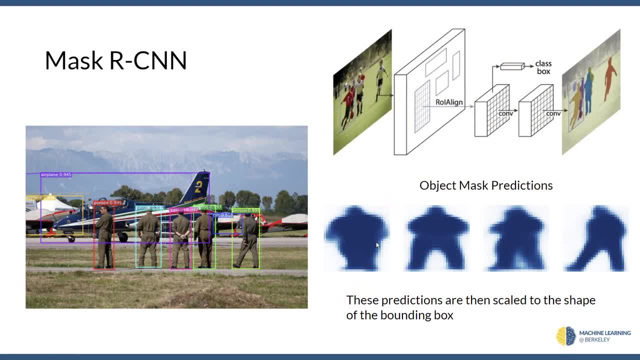 Right, Like these are correspondences and people. again they're scaled to the shape of the batting box because RCNN, But so you can see that those kind of are all working, and then they're scaled back up to kind of match the corresponding output And so, yeah, here's an example of this. 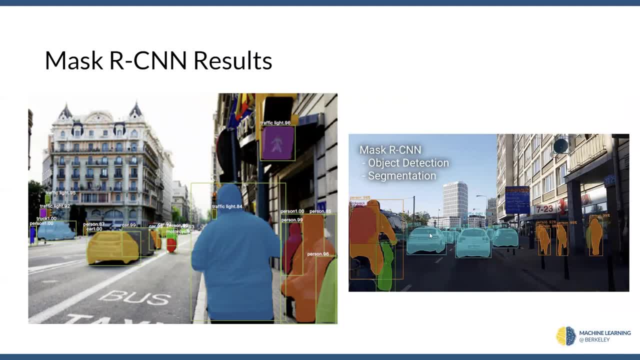 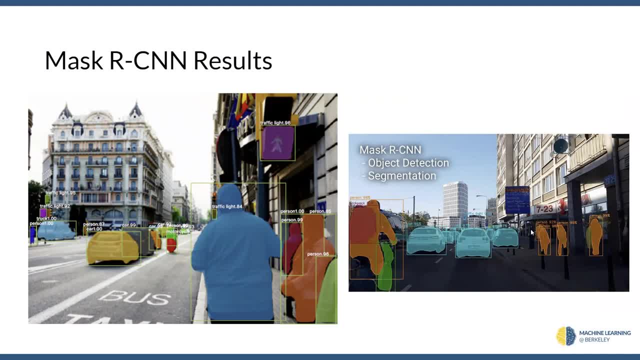 know like it's able to detect this backpack on the person as well as kind of identifying each of these different people's and each of these from cars as separate objects. Yeah, that's. I believe that's about it as far as the slides, I don't have any questions right now. 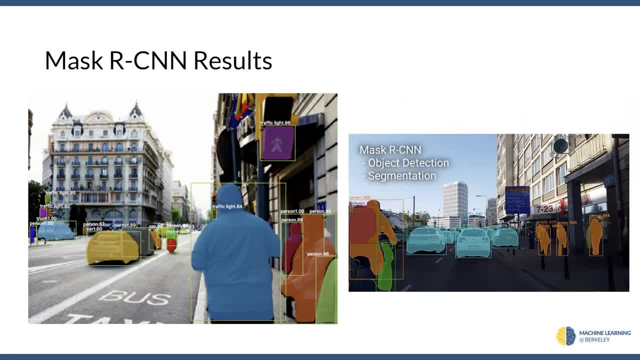 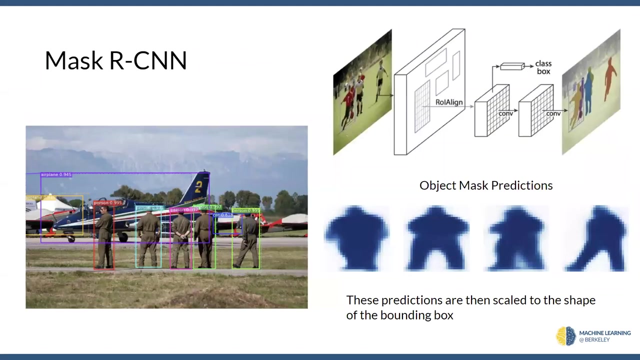 Yes, So I understand this Basically right now- some objects that you can classify and then you're going to find, like sometimes it's the same mutation everywhere. Yeah, you can kind of think of it as it's a little bit simpler because we have the 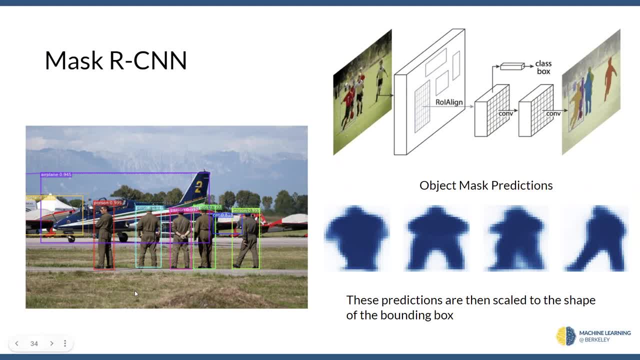 not that you have to remember all the details of this, but when we're doing RCNN, the, when we pick like a potential bounding box and try to classify, we essentially like, squish it down into like a certain size box And then we run the. 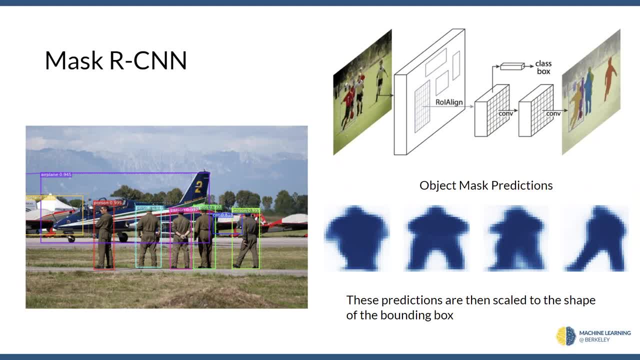 classification on it. So the idea is that we are guaranteed to have like a certain fixed size image, So we don't necessarily have to do like a fully convolutional. I think there's different kind of ways you can do that. But yeah, that's, that's pretty much it, Yeah. 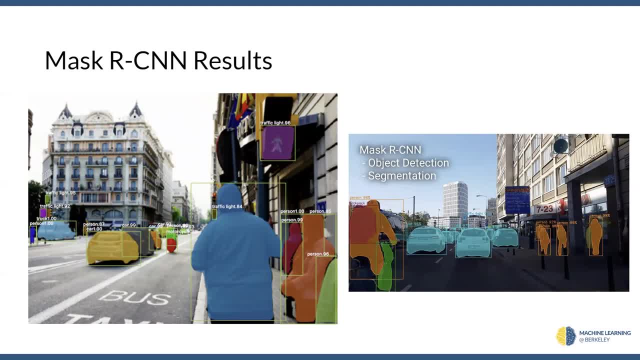 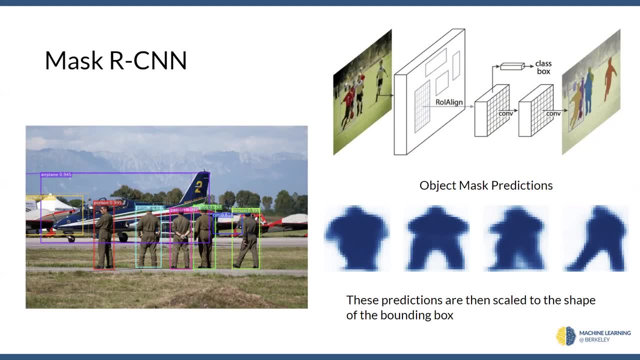 I don't know. Yes, What is the label? Oh, that's a good question. So you know, I'm not actually sure how they collect it. Do you guys, Jenny, you guys know how they collect data to train the segmentation stuff on? 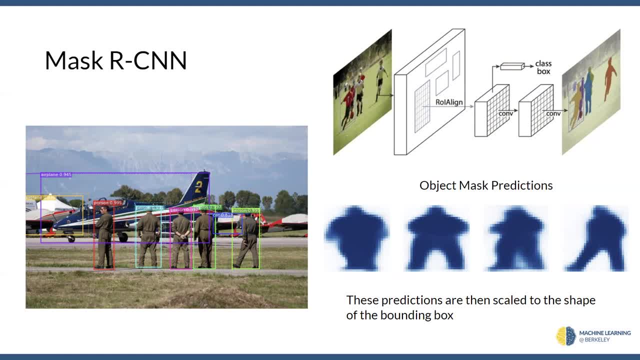 People are. for example, if you're labeled, you know you're my current tools and then that's your outline. Just keeping points on the principle that you can do: Yeah, that's one option. You just have people to do it for you. Just arbitrarily create the training data for you. 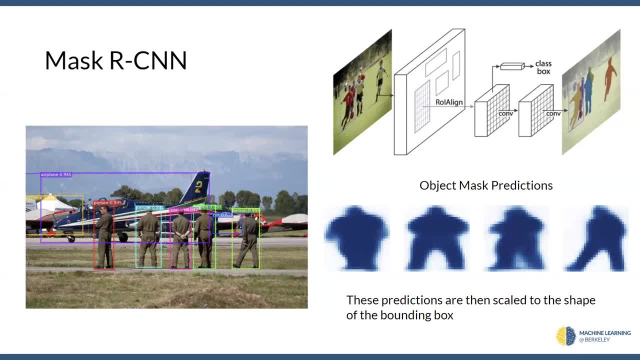 Okay, Yeah, Sometimes you do classic data system methods, or nowadays you can also be adjusting it to the initial values. You know, you're just going to adjust it a bit more. It's basically the same way. You know for classical: you find a way to turn it into different colors and it's the way. 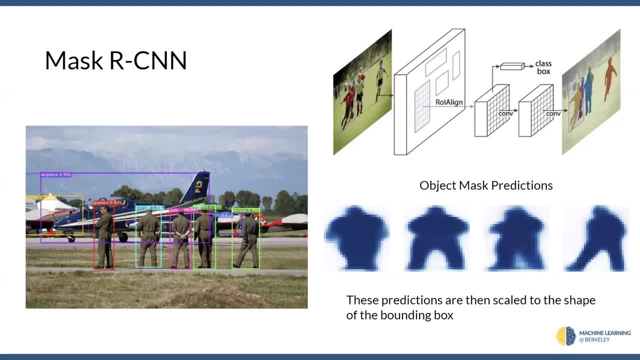 that you're trying to like form it and hold it together. Uh, it could also be phones. I cannot afford to adjust it. I guess I'm still, you know. Thanks, pal, Uh, does anyone else have any questions? Yes, 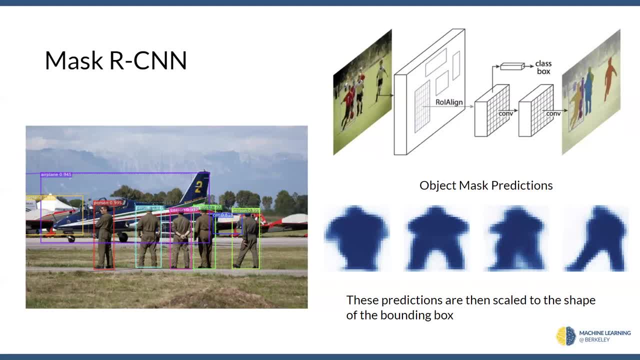 Um, how do you choose that? the user matrix for So that's learned, in the same way that you choose a filter for a convolutional network. It's just the weights, essentially. Uh yeah, Yes, I understood All right. How is the what? 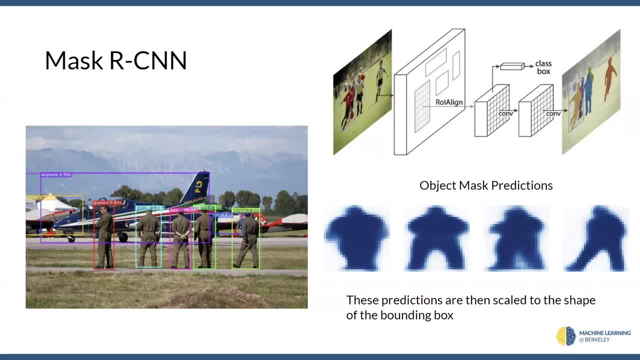 The deconvolution. Yeah, So I mean essentially, like it's kind of hard for me to answer that question without like, having a bunch of like labels and everything, But essentially it's like it's really just the exact process that I was talking about before, right, It's. 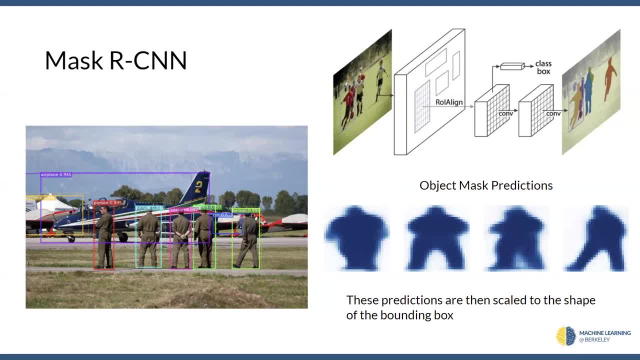 it's literally just a projection. You take the filter, you multiply each value in the filter by the uh you know value of that corresponding pixel or that corresponding uh slot, And then essentially, you know, you're, you're iterating your filter over the uh image. You're, you're. 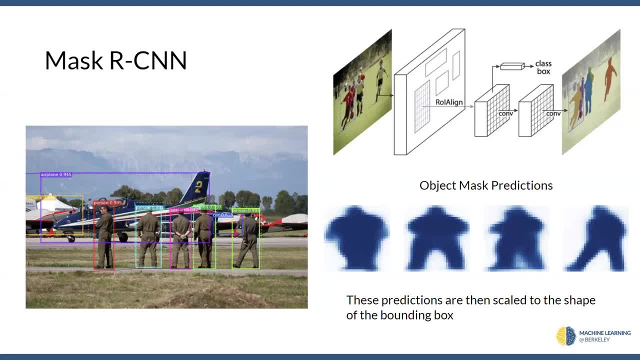 iterating your multiplied filter over the image And essentially at each point of the iteration you just add the spot at that corresponding filter to the spot in the output. Uh, and then you just kind of keep passing that over. Yes, Question was more of uh for convolution. it's like vector and major. 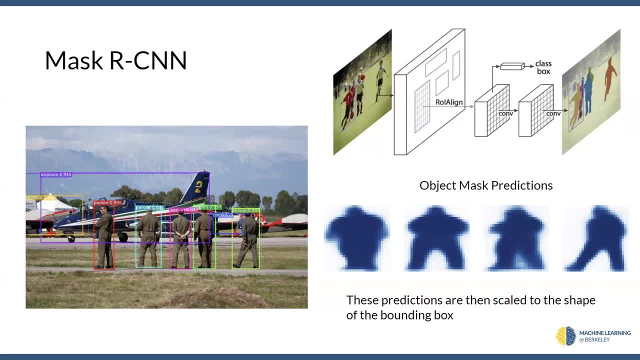 complication. but what's the equivalent for? Ah, You know, I can't actually remember. I can't actually remember off the top of my head how this is optimized. Um, I don't remember. I can get back to you on that one. Sorry about that. Yes, 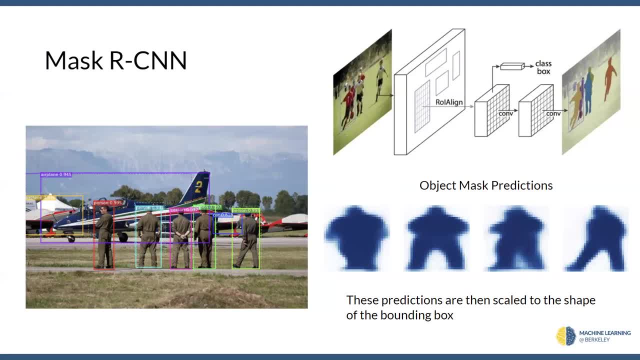 So not really. I know I presented it like that. Um, it's not actually like inverting a convolution, It's just easy to kind of think about that Like it's easy to think about it that way. It's not really doing like. 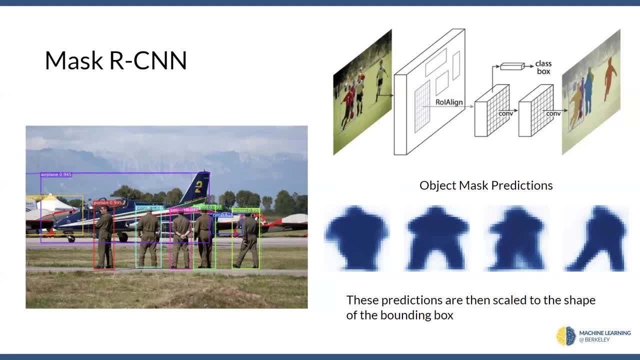 an inverse of like a convolutional operation. Yes, Yeah, yeah, Yeah. So between those, I call it a transposition, It's a. it's a bit hard to define that. It's more of a process. 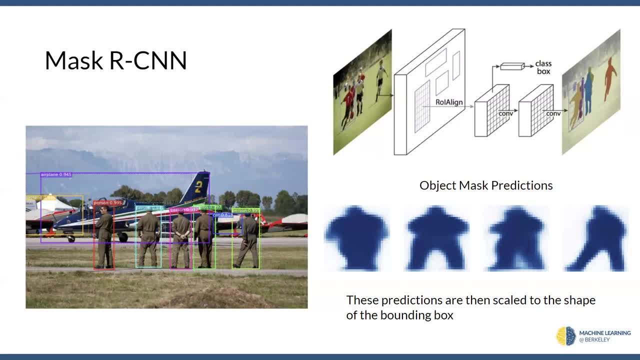 Yeah, I'm sure there are like formal definitions of like, like essentially efficient ways to optimize this. We didn't actually look into this for this class. Again, the point of this is not to like have you guys implement, you know, uh, like PyTorch, It's just. 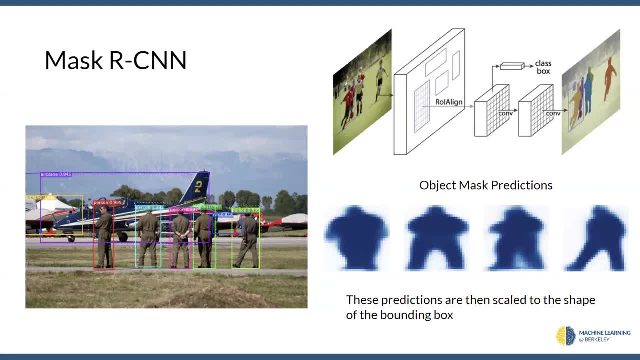 be able to like understand, like conceptually, what this is doing and then just trust that the people who wrote the algorithms implemented it in some fast matrixy way. um, that I actually don't know. I just don't know off the top of my head. Uh, but yeah, Any other questions? 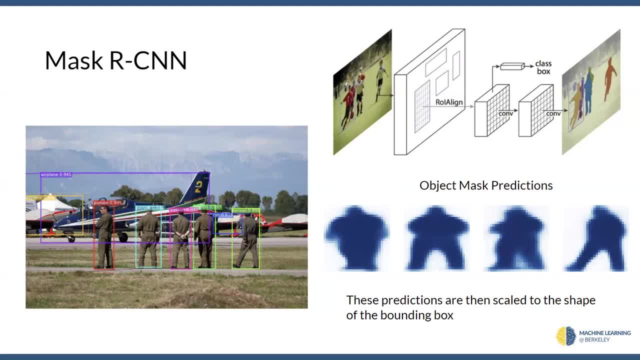 No, Okay, great Rohan, do you want to show the demo? Yeah, I said you could sign one for the one. Okay, okay, Yeah, yeah, Let me One second. I'll blank this real quick, just so I can open up the. 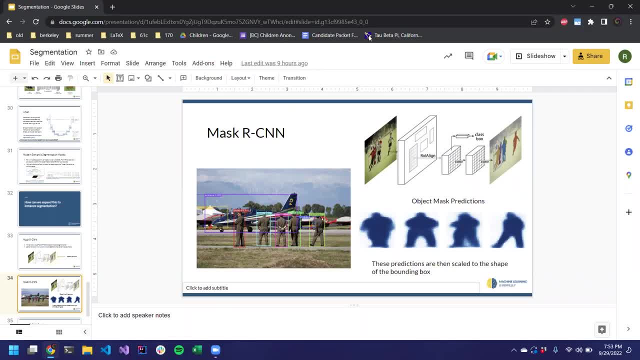 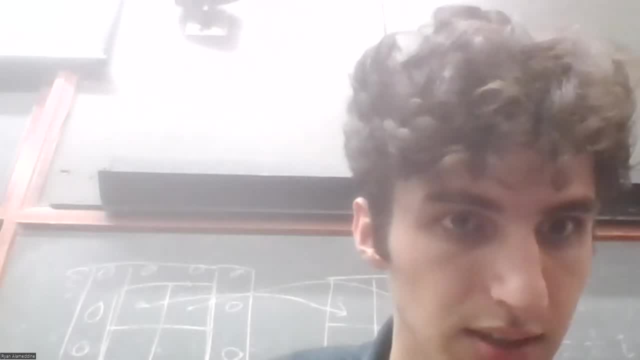 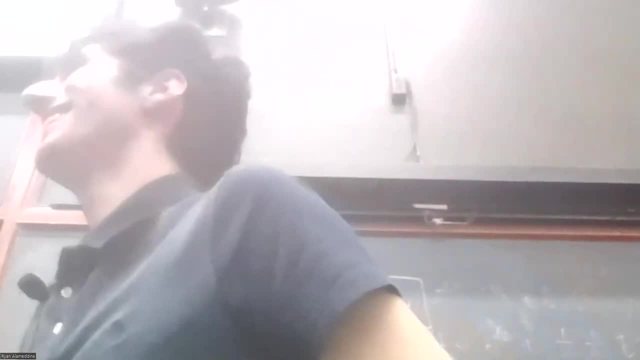 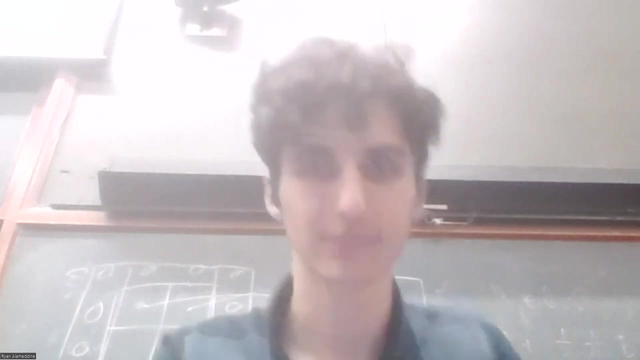 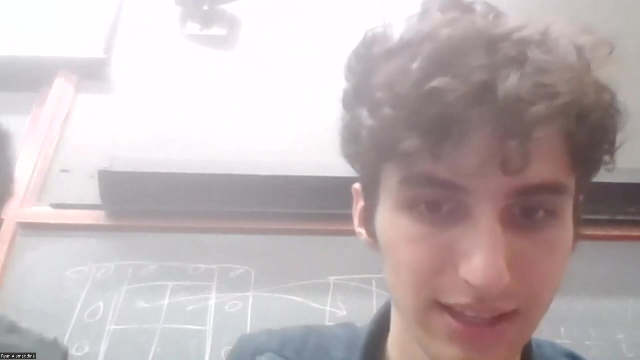 Wait, sorry, Which one? Can you, Oh, set semantics like tiny URL. Uh, okay, okay, Should you just be able to run this. All right, let me. I stopped screen-sharing. I'll give you one second. Uh, can you walk through it? 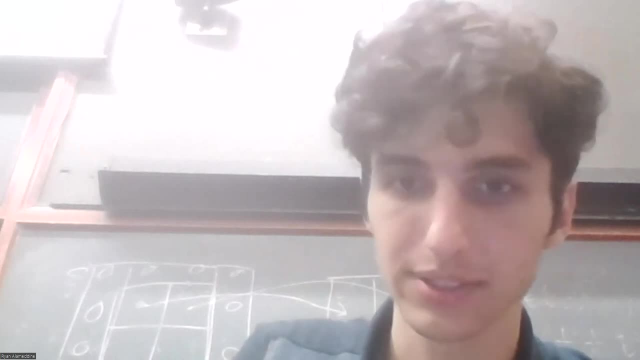 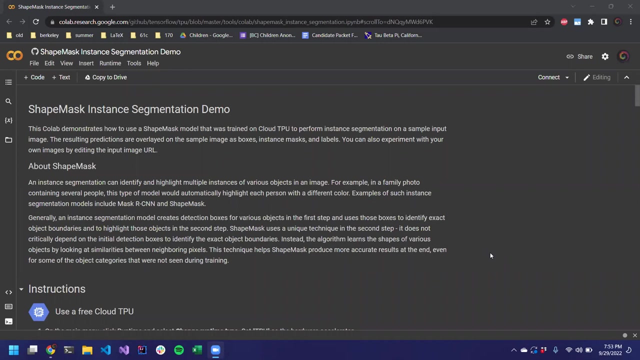 Let me screen-share again. All right, perfect, I can give you a moment. Do you want to like? Oh yes, So yeah, This is just a quick demo of a trained model that was trained on Cloud TPU. This is an. 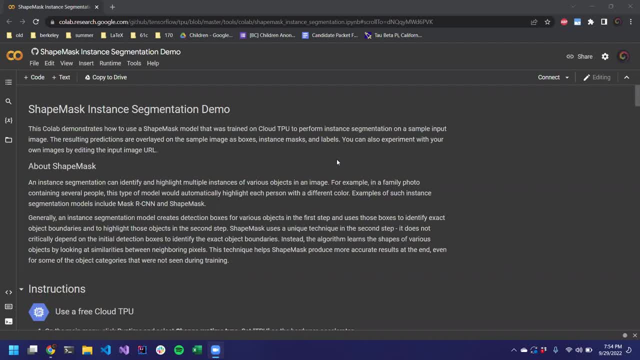 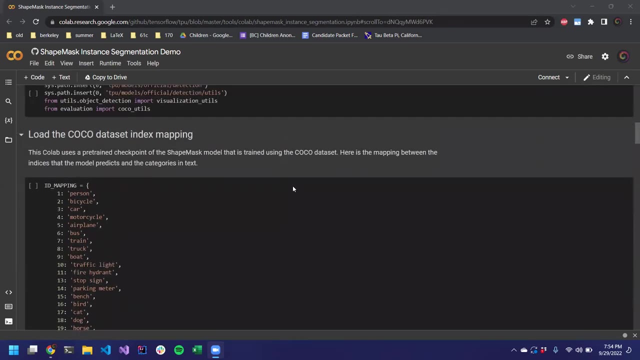 instant segmentation model, So literally all the details are abstracted away. This is just like a visual representation of how instant segmentation would look post-implementation. So yeah, we don't even need to run this. Essentially this: the Cocoa dataset has a bunch of IDs. 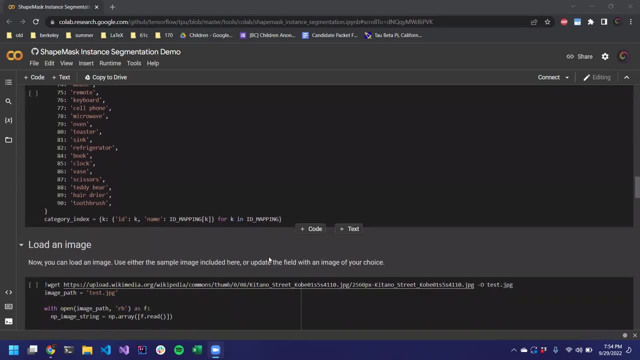 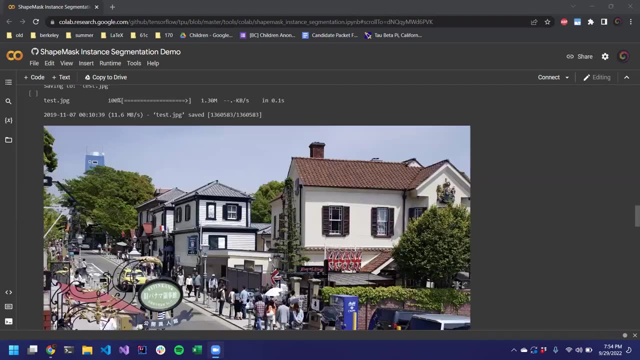 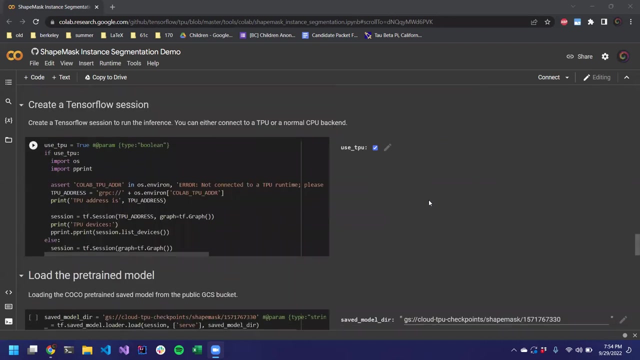 This is just a map of all of those. to re-associate what the segmentation model says to whatever it's like. ground truth label is: Yeah, so this is the image they passed in. I think this is somewhere in Japan. All of this is literally just calling the model that has been pre-trained. 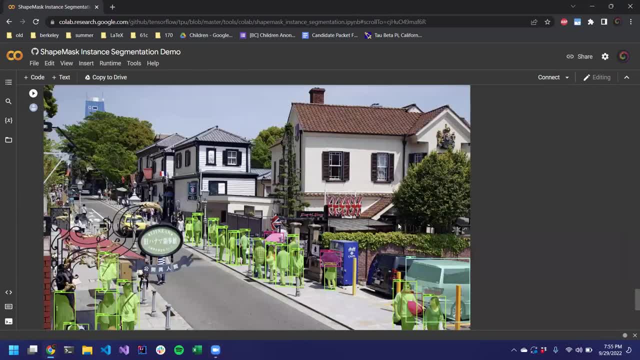 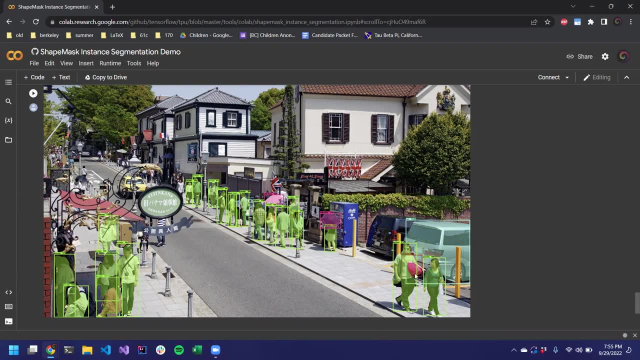 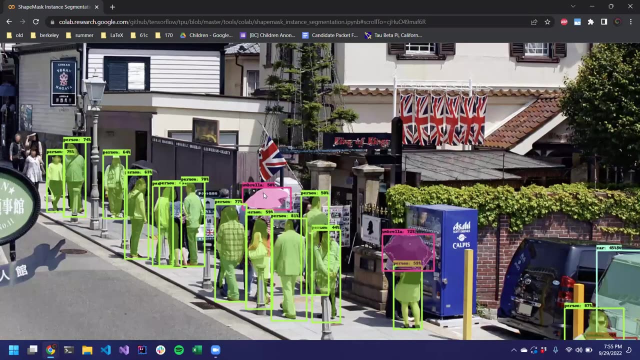 This is what I wanted to show. This is an example of instant segmentation. As you can see, there are multiple people that it's detecting in various capacities. It's also able to detect things like umbrellas with a 50% accuracy score. It's a little more secure on other 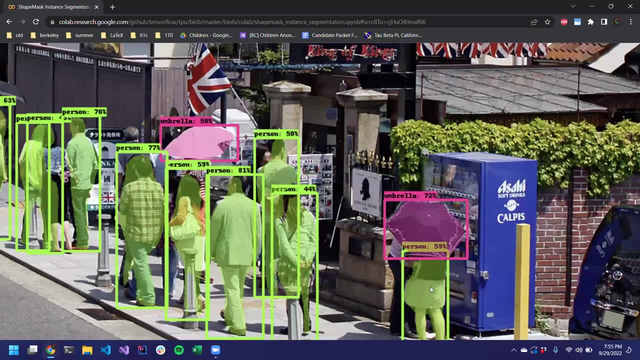 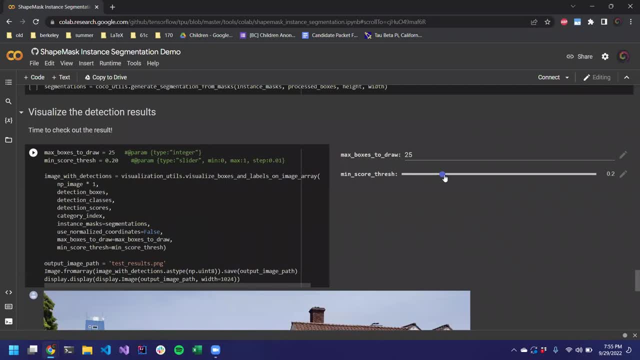 things. As you can see, it looks like there are two people behind this umbrella. It was not able to get the second one. What's interesting about this model is that you can give it a score threshold to predict on. You can also visit the URL for this. 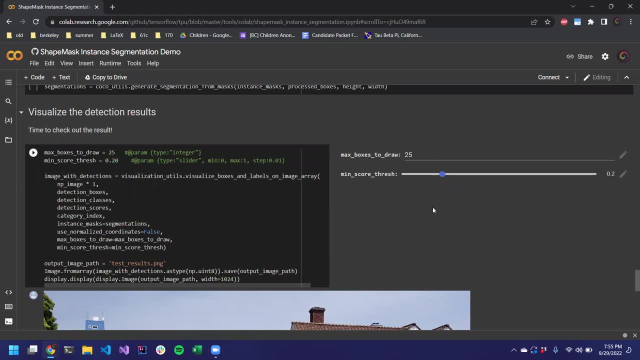 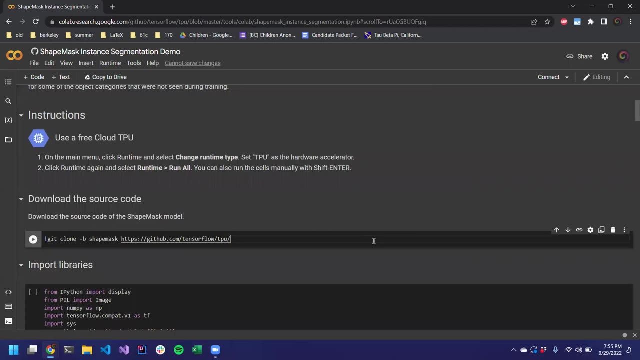 It's tinyurlcom slash semantic dash seg. Then you can actually play around with the parameters. If you were to increase this to 70, a lot of the Actually maybe running through it isn't a good idea. You'll post a link on it. Yeah, We do have a little time. 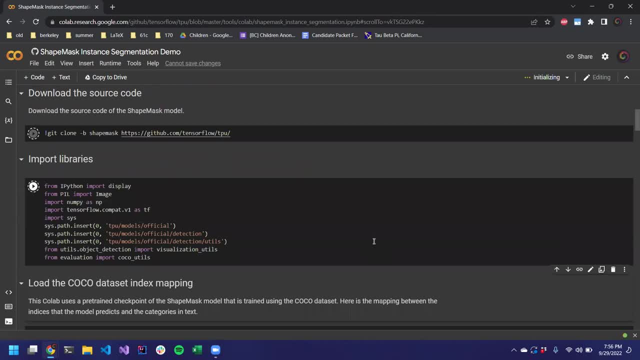 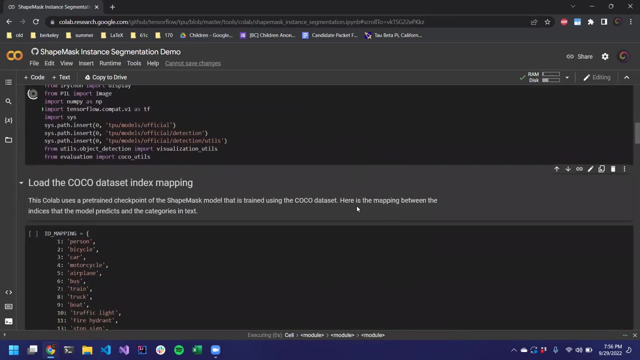 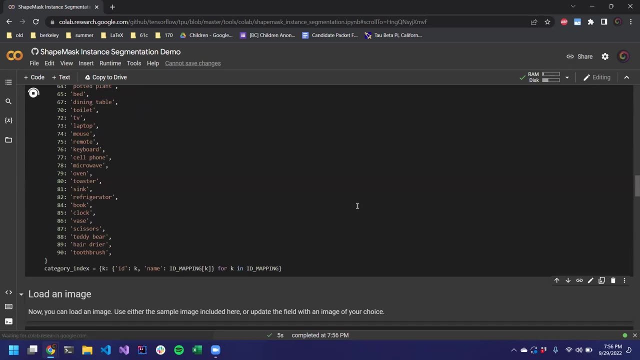 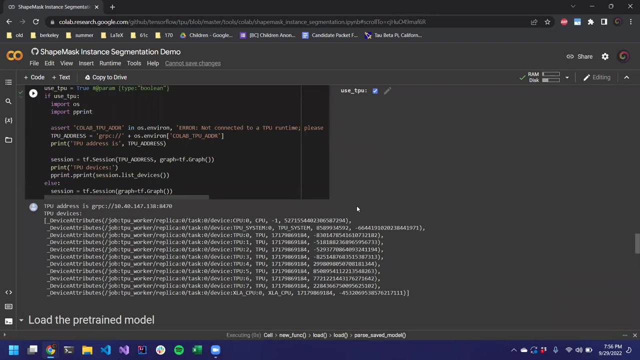 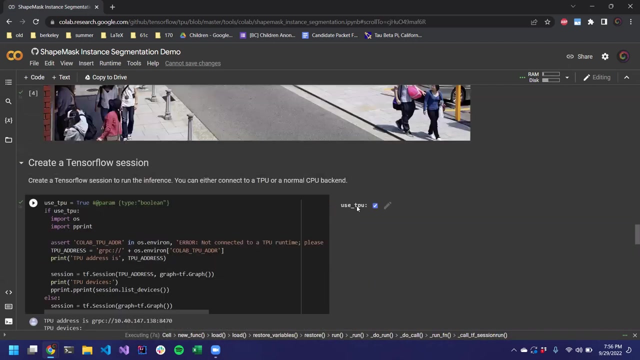 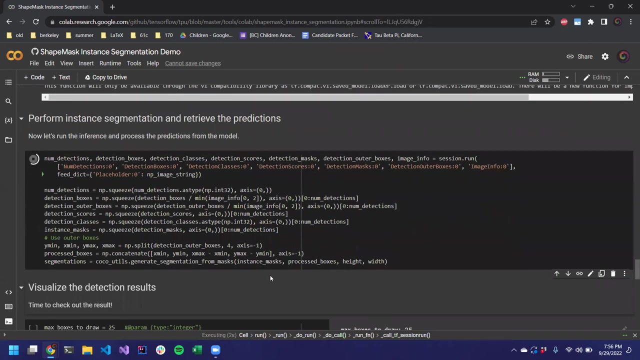 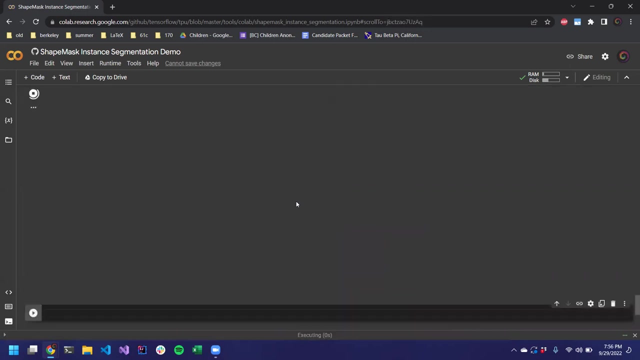 If you guys want to follow along: tinyurlcom slash semantic dash seg. If you guys want to follow along: tinyurlcom slash semantic dash seg. If you guys want to follow along tinyurlcom slash semantic dash seg, All right. If the min threshold is increased, you're only accepting information where you have 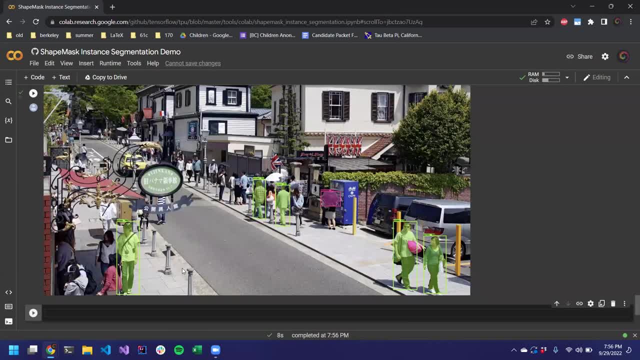 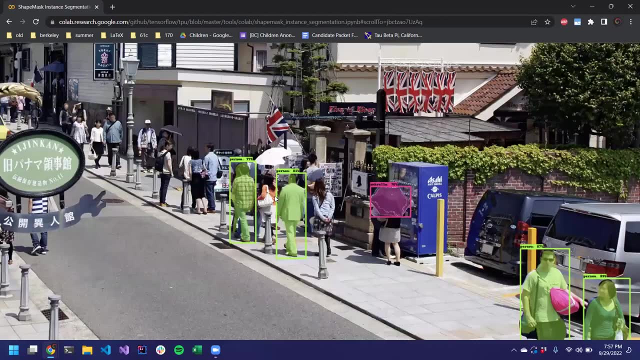 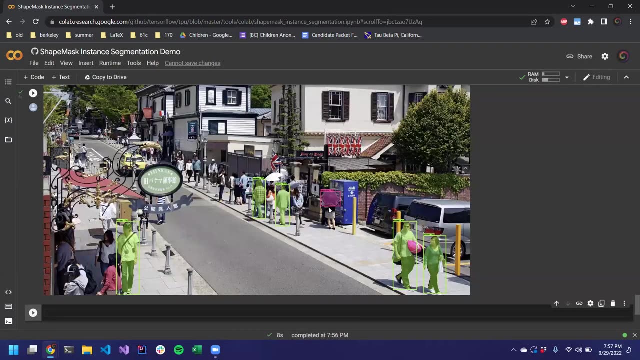 a very high likelihood of the semantic segmentation being accurate. As you can see, the handbag goes away. All of these people go away. The only people that we see are things that the model can very confidently say it can draw a bounding box around with over 76% accuracy. This umbrella is 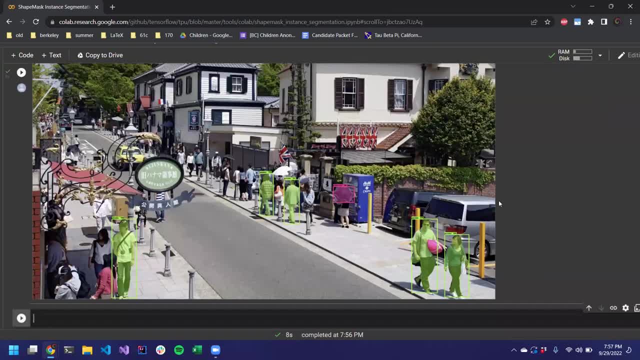 exactly on the boundary: The pre-training. the beauty of this model is that you can pre-train a lot of things on the cloud on AWS- a lot of offloaded services- and bring them together in a notebook like this. Your homework is going to be a lot easier. You're going to be able to do a lot of things on the cloud on AWS- a lot of offloaded services- and bring them together in a notebook like this. Your homework is going to be a lot easier. Your homework is going to be a lot easier. You're going to be able to do a lot of things on the cloud, on AWS, a lot of offloaded services and bring them together in a notebook like this. Your homework is going to be a lot easier. You're going to be able to do a lot of things on the cloud, on AWS, a lot of offloaded services and bring them together in a notebook like this. Your homework is going to also be a Collado notebook. 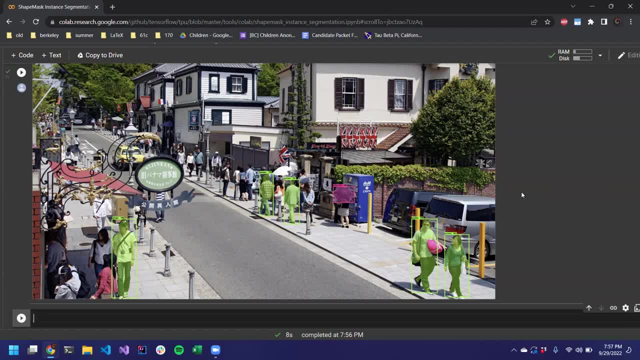 I believe ResNet assignment is mandatory and U-Net 1 is optional, but I would highly recommend doing U-Net 1.. I think a lot of it is done for you and RA can talk more about that as well. So feel free to come to Office Hours if 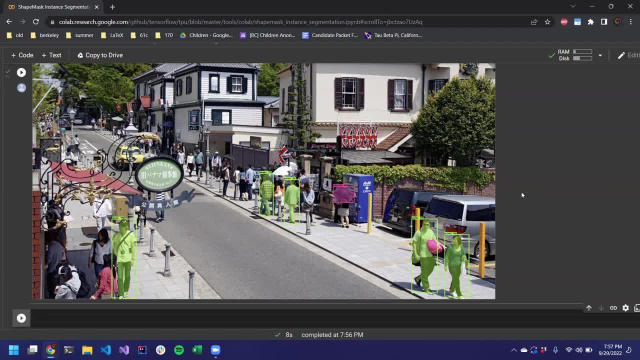 you have any questions about that? Oh sorry, That is due- I think it's being released tomorrow night. Okay, it'll be over a week from now, So- And it's also everything is on the course website, So all the due dates and assignment links will be there.